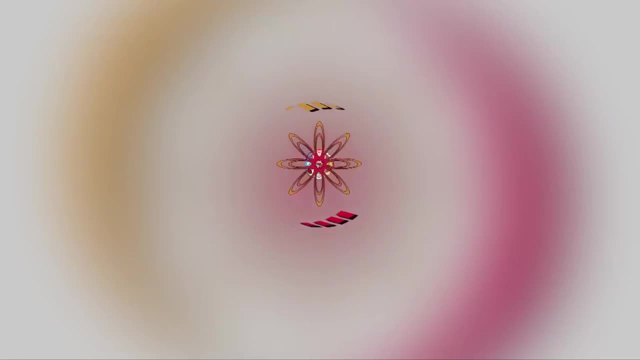 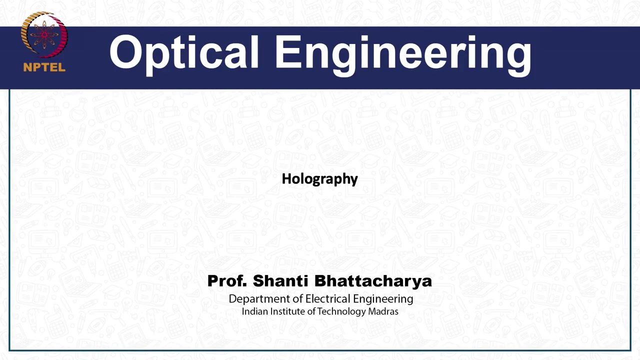 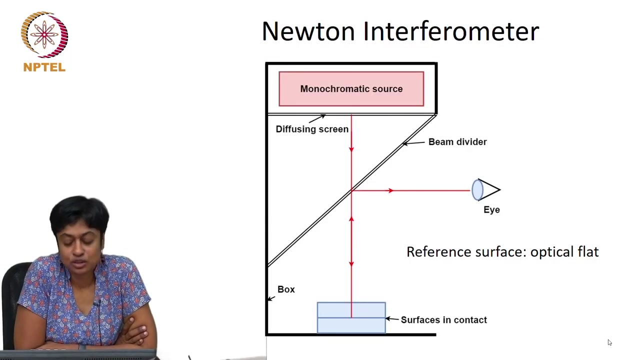 Good morning. So we were looking at the applications of interference last week and, in particular, we were looking at using it to test surfaces, right? So, just to refresh your memory, I have the Newton interferometer here and, as the name interferometer suggest, it will create 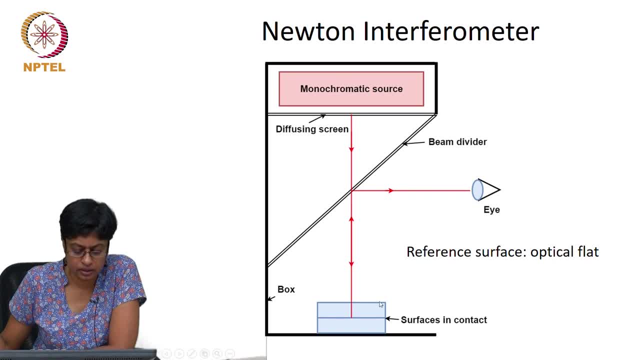 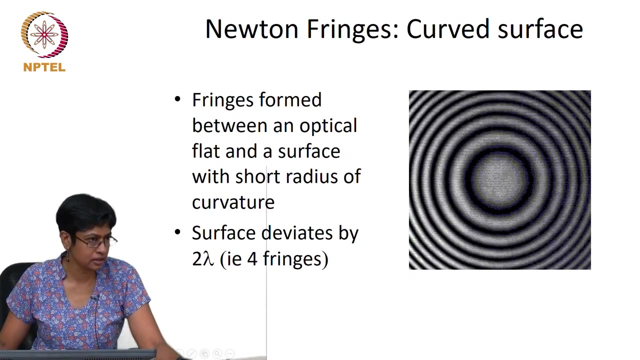 two beams. The two beams that we are creating is: one is the reflection of the top surface of the device that is being tested and one from the lower surface over here, and we saw some of these images. So if you had a convex surface, for example resting on the reference flat, you would get 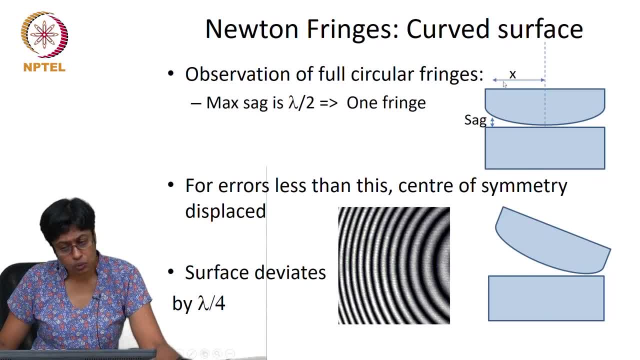 fringes like this, and you could not only check what is the nature, what is the shape of that surface, but you could also get a quantify. you could also quantify how much is the curvature by counting the number of fringes, and if you had a very low curvature, So that you did 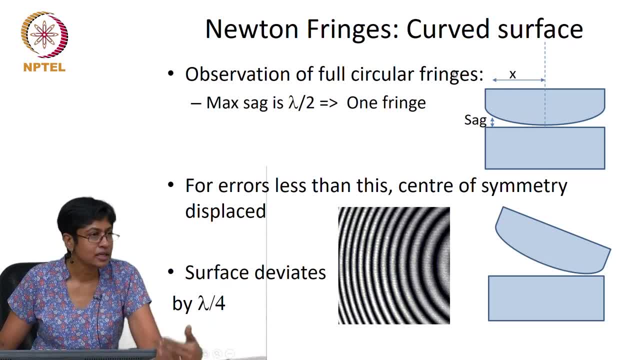 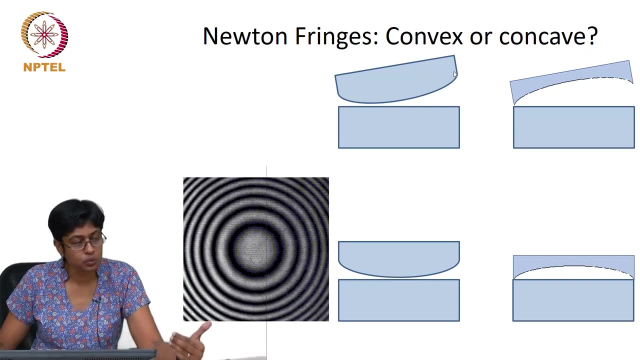 not have a full fringe. you could tilt the device So that you create more fringes and use that to help you quantify the curvature. Then we also looked at how do you tell the difference between a convex and a concave structure, and that would be based on how the 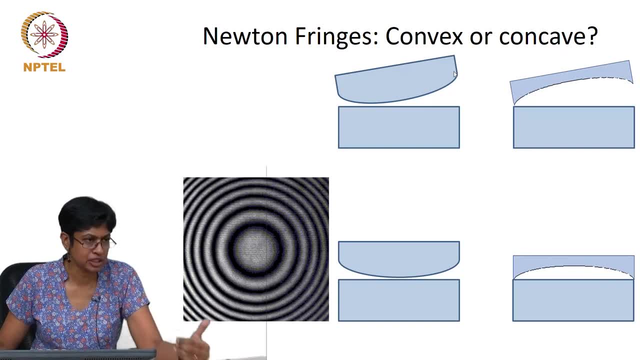 fringes move depending on how you apply pressure to the device under test. ok, So main point you should have got from yesterdaynell. Let us get deep diving there. These are the put yesterday. last week's lectures is that interference very quickly gives you a visual on the shape. 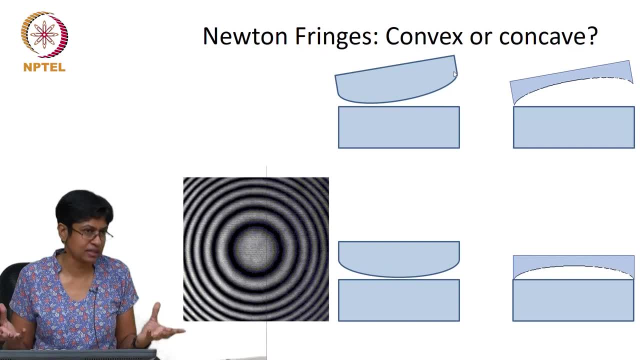 or it could be the shape or the refractive index right. So it gives you a visual on the optical path length difference between some test object and a reference object, and the main idea to get is your always introducing a reference which, whose sole purpose is to 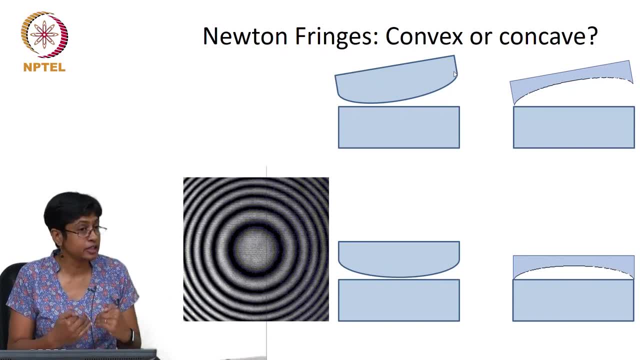 allow the interference to happen. So the idea is you have a reference that is known. does not matter if it is a plane wave that is tilted, if it is a spherical wave, it is a diverging wave, really does not matter. the point is you know everything about that wave. 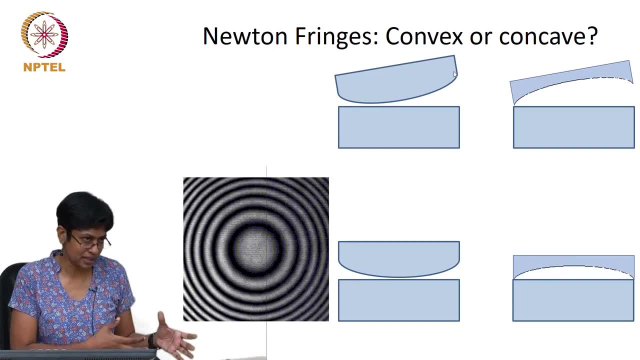 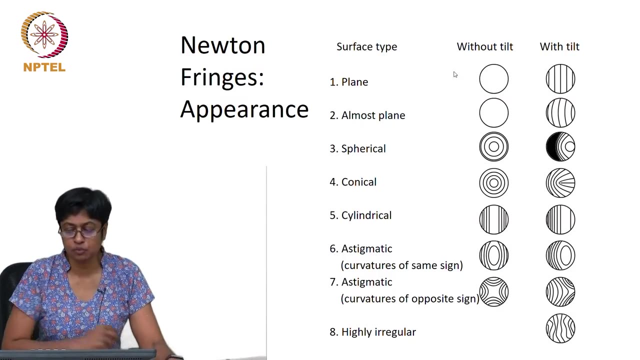 and you are interfering it with a wave you do not know anything about. but from the fringe path pattern you can extract information about the unknown. that that is the idea, ok, So today I want to move on. oh yeah, before I move on, just to show you typical fringes. 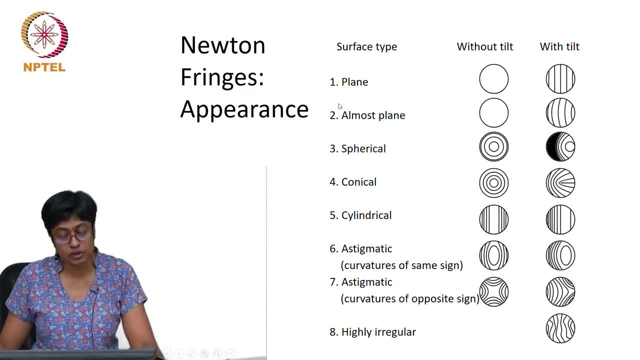 you get with the Newton interferometer for different types of surfaces. So if you think back to our very early geometric optics days, we had wave. you could think of the wave traveling through your system. we looked at rays and we looked at ray pictures or intercept curves. 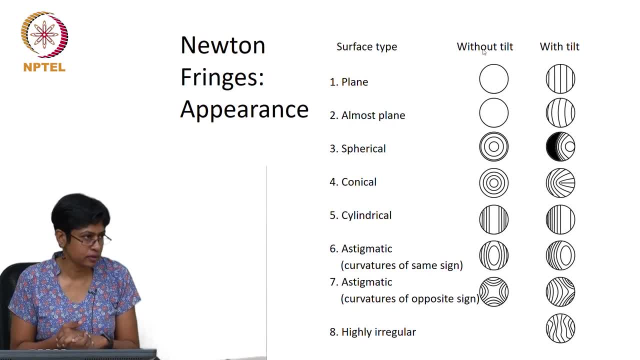 to tell what are the kind of aberrations we had in our imaging system. But you could also look at a fringe pattern and the fringe pattern between a plane and a plane reference wave and the wave of interest that the fringes would tell you about the 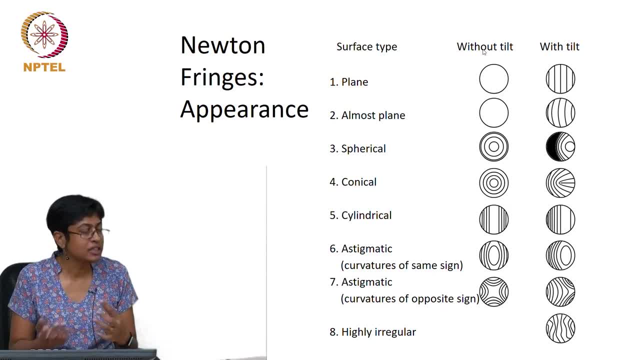 wave front, the shape of the wave front, and if there is an aberration in that wave front it is going to be obvious in the fringe pattern. ok, So if you look at the list of surface types here, it this could mean this is my surface and I am. the wave is now reflected off this. 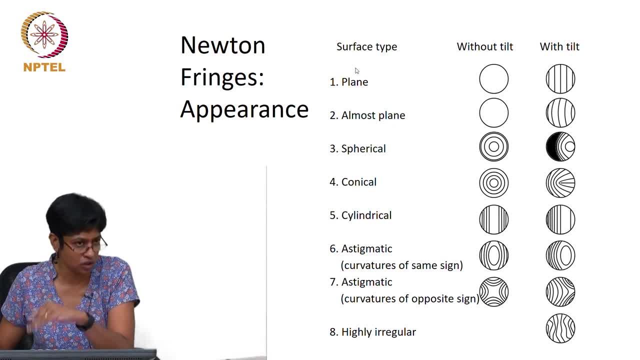 surface. So the wave now carries this information of the surface. I could also just think of it as the wave front has this shape and I am interfering it with another wave front and therefore I am getting certain fringes. Now, if the two beams that are interfering 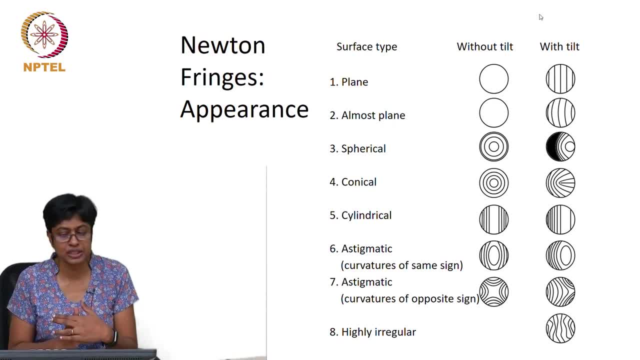 the reference and the beam from the surface of interest. there is no angular tilt between them. they are perfectly in line. in the case of the plane wave, we know that you are not going to see any fringes at all. we discussed this case with the Michelson. 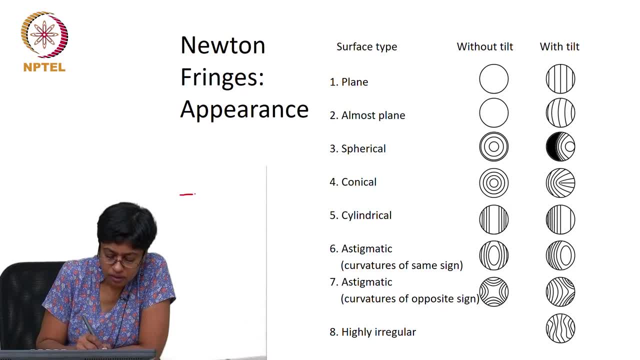 So we said in the Michelson: you have a beam coming from source, you have a beam splitter, you have a mirror, you have another mirror, and if these two mirrors are perfectly perpendicular to each other, the wave fronts coming from them are going to have a equal spacing between. 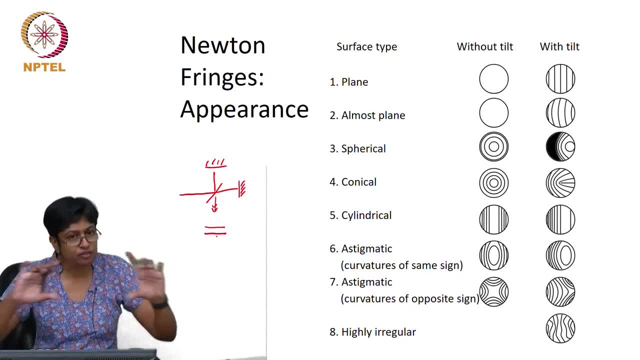 them And since the spacing is everywhere equal between them, you are not going to see fringes because there is no difference in path length. you see constructive or destructive interference because of the change in the path length. If the path length is the same everywhere, I am not going to see that. So if I do not have any tilt and the reference, 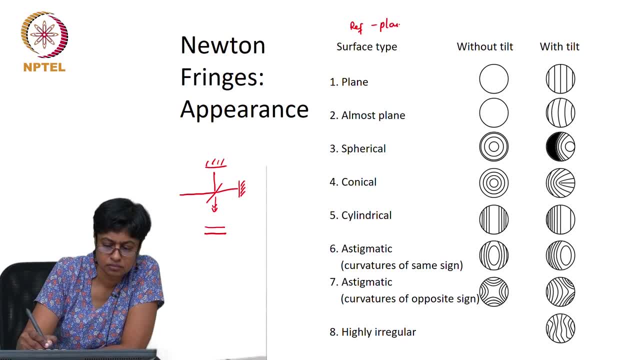 here is assumed to be a plane. it is a plane wave. So if I have two plane waves, there is no tilt between them. I am not going to see fringes. So it is only useful to me if somehow I introduce a tilt and I see these fringes. If it is almost plain, it means the 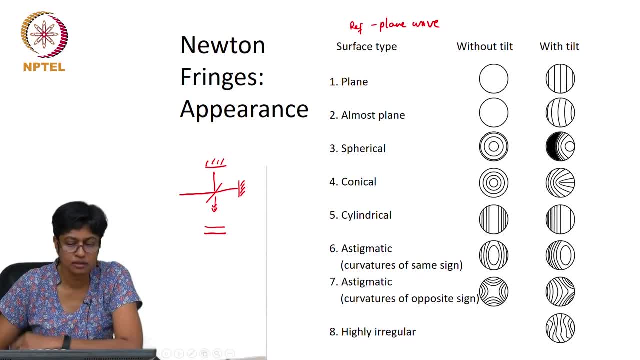 fringes are going to deviate slightly from those linear case as is shown here and, of course, if it is spherical, as we saw, you will get the rings and for different shapes you can start seeing how the fringe pattern varies. So this is a visual way of quickly seeing. 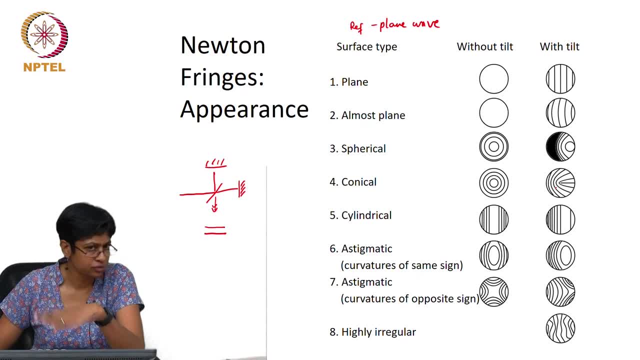 how aberrated your wave front is or, if not aberrated, what is the shape of the wave front. ok, So very quick interferometric technique to do that and because you are looking at the reflection of from the surfaces, from the top and the bottom of this element under test. 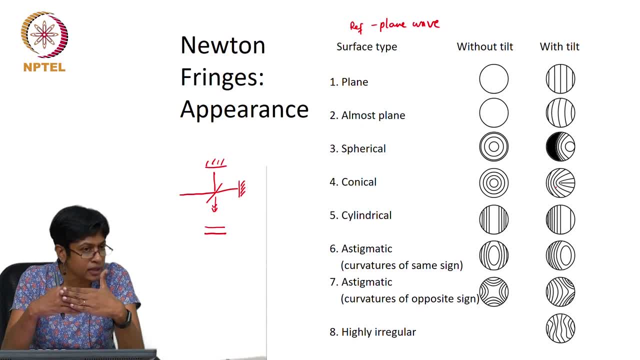 the path length is very. difference is very small, So you do not have to worry about coherence length. the source that they are using, its coherence length will be larger than this and there is no alignment that you need. Have you done a interference experiment? Even B Tech lab will have Newton's rings. you 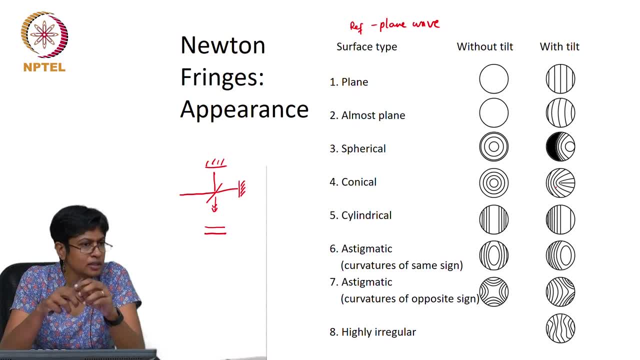 will have Newton's rings right. Do you put it in and you see the fringes immediately. You have to look carefully. do something. Newton's rings should be fairly straight forward. Have you done a Michelson interferometer experiment? Did you get fringes immediately? 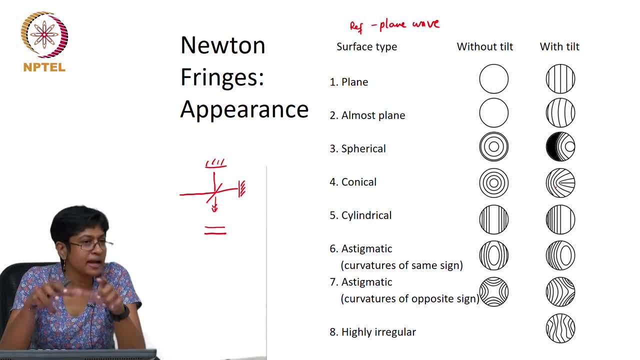 No, Right. So when you have this different path lengths, then you have to match the path length quite carefully, even for a source with the good coherence length right. So you, whenever your set up is such that the paths are the same, the interferometer is a common path. 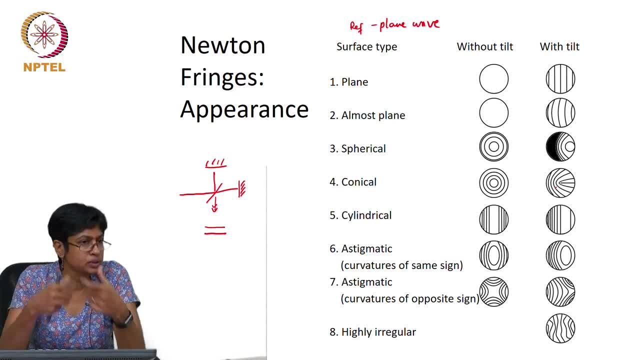 interferometer. It is much easier because you put it in and there is no alignment right. So the Newton's is a very powerful interferometer because it very quickly gives you information and it is. there is no alignment needed So early on a workshop, in an optical workshop it would. 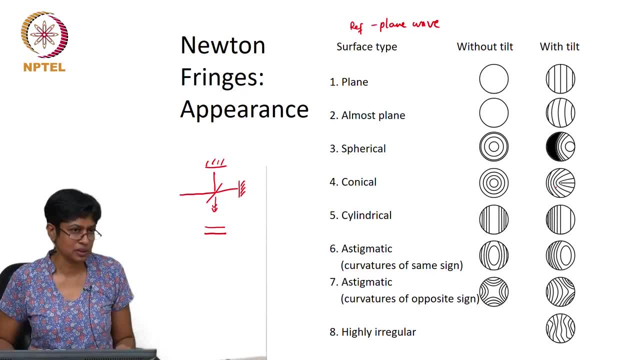 be definitely a tool that everyone would be using. ok, So with that we end the one part of using interference for testing. but the applications or the possibilities that exist using interference are huge. There are so many things you can do with interference. You could- I could run an entire course on interference. I am, since 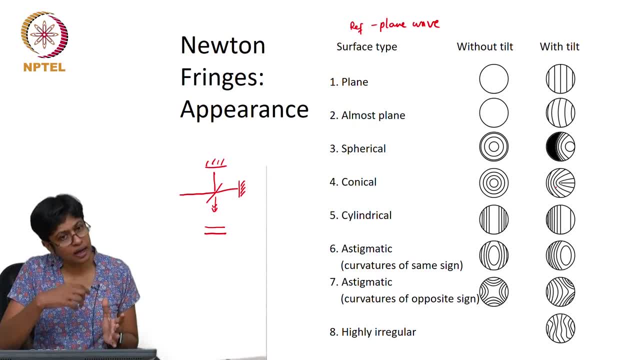 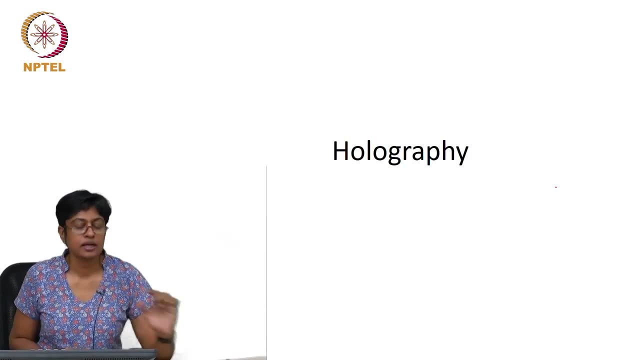 you only have a few classes. Ok, What I want to take you to one other idea that is used in a lot of different applications, but I am going to show you the idea and then we look at a couple of applications of that idea. So this is the idea of holography. ok, How many of you have seen a hologram? You? 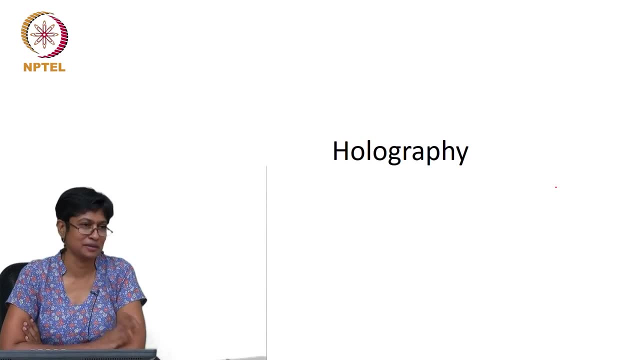 have all seen a hologram. ok. The answer to that question is: you have all seen a hologram. Where have you seen a hologram? Certificates, Certificates- ok, That is the first thing you think of. every day you see a certificate. 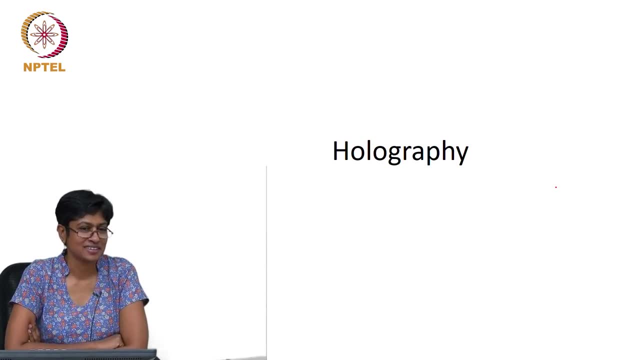 where else. Lot of products nowadays will have a hologram stuck on it. Why? Because you want to show that it is a genuine product, and if you just put a sticker that says this is a genuine product, you might find that it is pretty easy to print such a sticker. 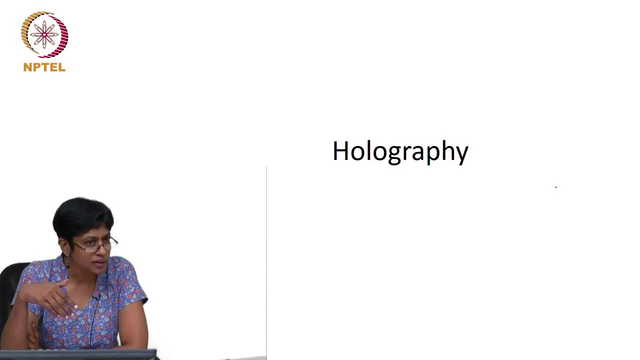 Ok, Whereas a hologram is not easy to make, So the belief is that it is harder to make a hologram and therefore that is a good thing to use on a security device. A lot of currency notes in the world which have holograms on them and they are used in a variety of places. 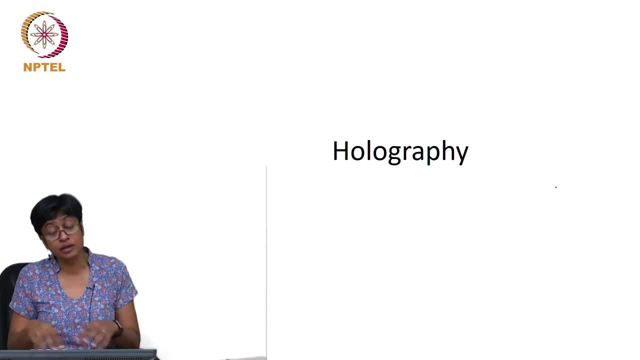 as security device. They are used because you can see- now you have to holography. you can see that holography uses interference. So you, it is not a simple matter of taking a photograph or just taking a picture of something. you have to set up and create this interference. 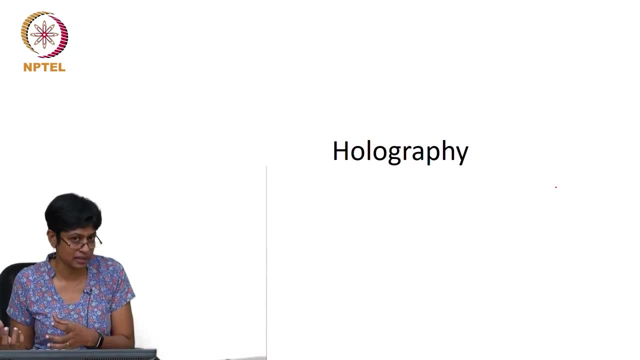 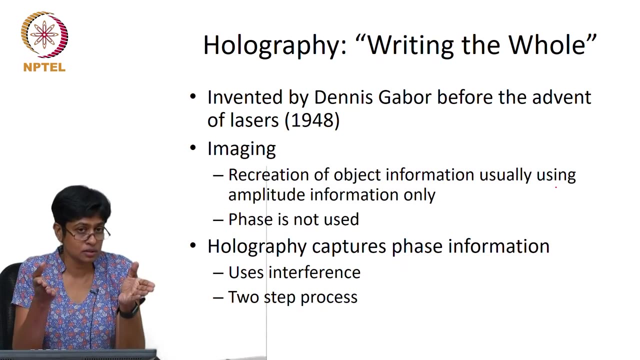 pattern and somehow create the hologram out of that. ok, Now what is holography For all of this course, we have been looking at designing systems or looking at the optics of systems. Some examples talked about imaging systems. So in an imaging system you took some optical. 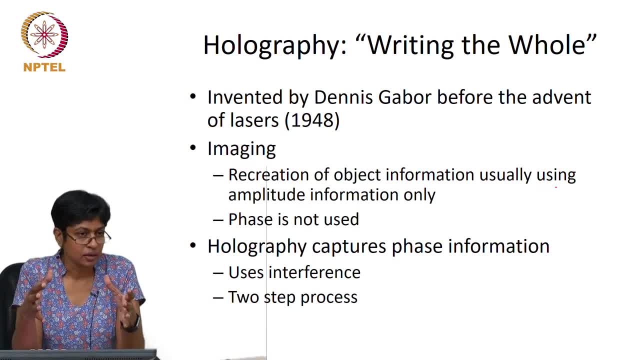 system and created an image, What we may not have explicitly said, or at least not every time. I said we took an image. what we were really doing is looking at the intensity variation. right, That is what a standard camera will do. we look at the intensity or the color variation. 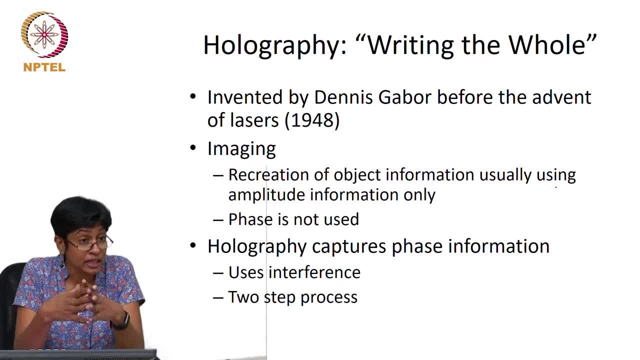 It tells you nothing about the phase. but, as you should now know, phase carries a wealth of information and, in fact, if I want to get true depth information, intensity is not going to give me that If I see a picture which has only an intensity variation across it. 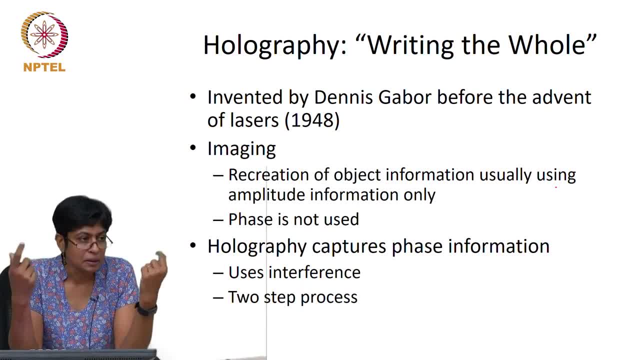 is a lot of processing that happens in my brain, based on prior experience that feels than in the depth information. So I know what the depth information would have been, but that is not giving me something I can quantify. And in a case where I do not know what to expect, I am looking at the images of some 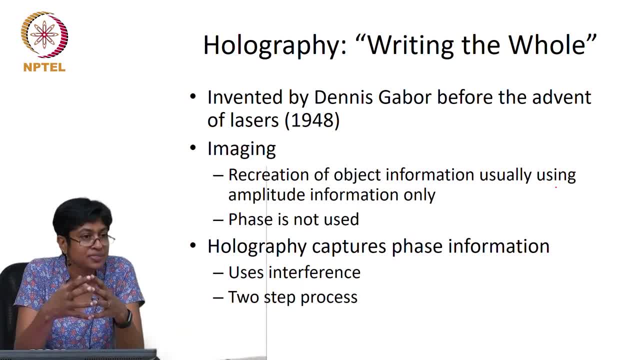 cells. I do not know what I am supposed to see. then I cannot look at a pure intensity image and really be able to tell anything about what I am looking at. So holography: It was invented well before the laser and it was thought: well, this is interesting. but 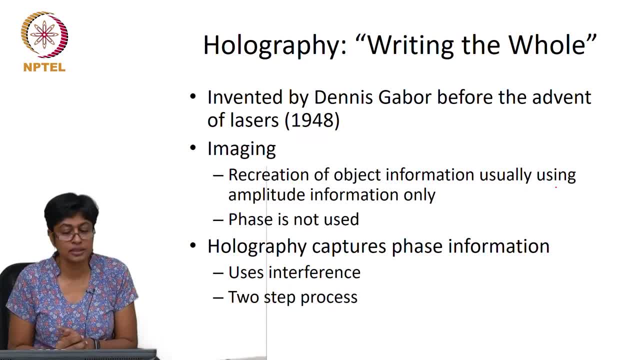 so what? ok, because it was not very useful at that stage. It does not only recreate the intensity, it also recreates phase. In other words, it means you get the depth information. ok, very, very crucial. It is a two step process, unlike the use of a camera, which, well, you might have thought. 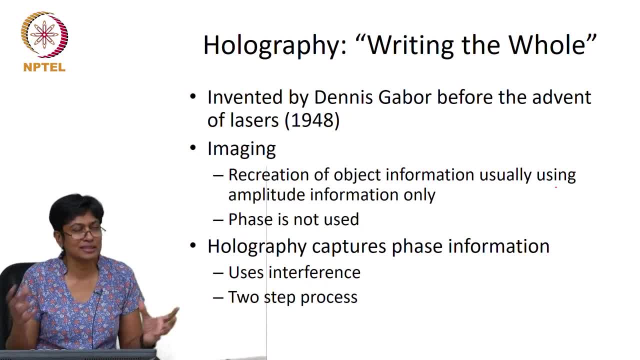 earlier camera was also two step because you have to take on multi step because you took a photograph, you had a film, you had to process and so on. But nowadays, with the digital camera, you take a photograph and you have an image, but in 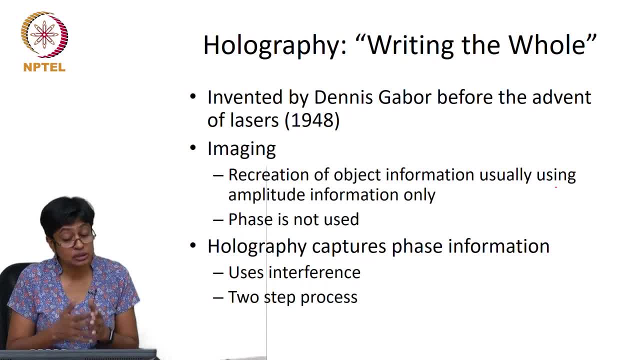 holography. it is still a two step process, because you take an image and that image you take is not a direct image but is an interference pattern. So you have to somehow record that pattern and then creating the image is the second step. 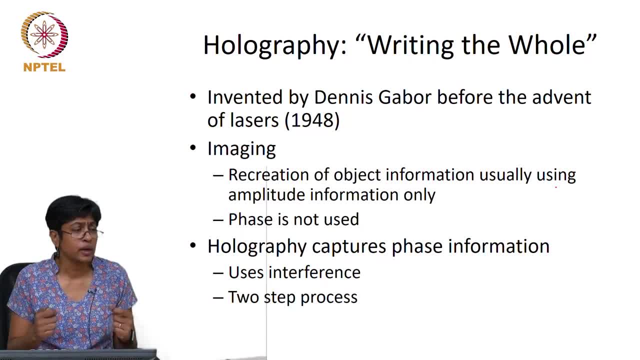 Which is called reconstruction. When you see holographic stickers on, you know, used as security or as to show something is genuine. what you are doing is the second part. you are using white light, ambient light, for the reconstruction process. Somebody else is carried out that initial recording process and somehow store that information. 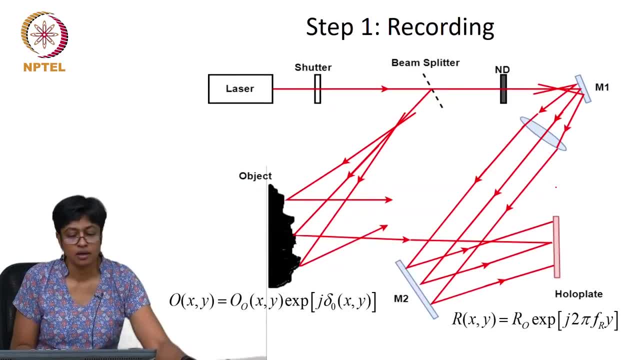 in that sticker that you are looking at. ok, So the first part, the recording part, it is. since it is an interference based technique, you will have a source with a good coherence length, So like a laser. I will talk about why you have a shutter later. 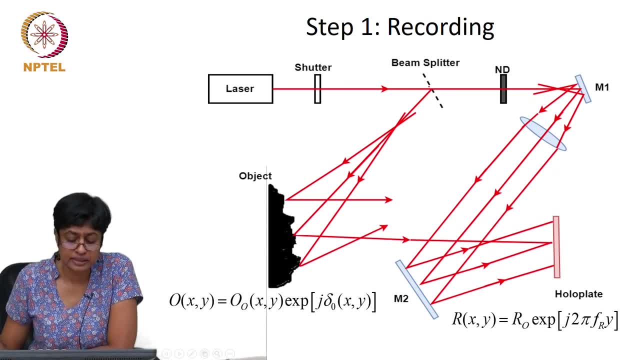 So you have a beam splitter which will redirect some part of the beam to an object. I am not showing you all the optics in this, So if you needed, the directions are shown by these lines. But if you needed the object, if your object was large, of course, you will use appropriate. 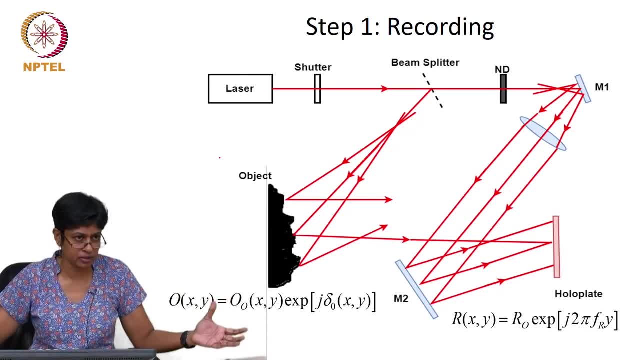 optics so that the light illuminates the object, just as with the camera. if you have not illuminated it, you are not getting back that information. So one beam goes to the object and scatters off this object. the scattered light now carries the information of the object. that is the information you want to somehow store and 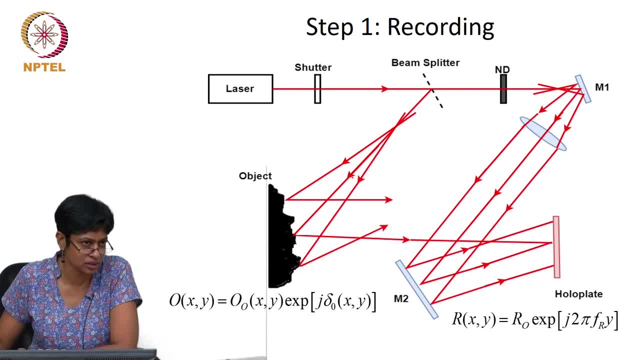 then later extract through the reconstruction process. The other beam goes to another mirror- I will come back to this element later- and that mirror. just, you have a set of optics, a set of mirrors and lenses that gets it to the correct size as well as redirects it to a plate which is sensitive to light, which is called the hollow. 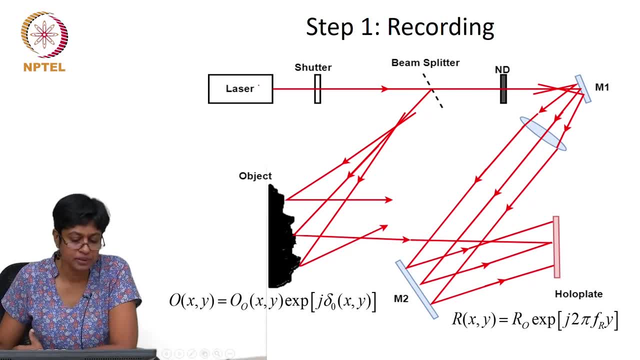 plate here. ok, So these are the two beams. Now there is one beam that acts as reference. it carries no information. all it does is travel a certain optical path length and arrive at this plane. And the second beam goes to the object. it reflects, of the object it carries the information. 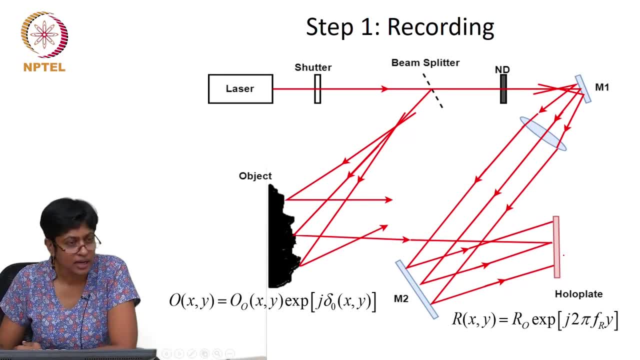 I am interested in and that scattered light arrives at the same plane. So what happens at this plane is an interference if you have set up your system correctly. The hollow plate is the substrate which has a material on it which is sensitive to light. 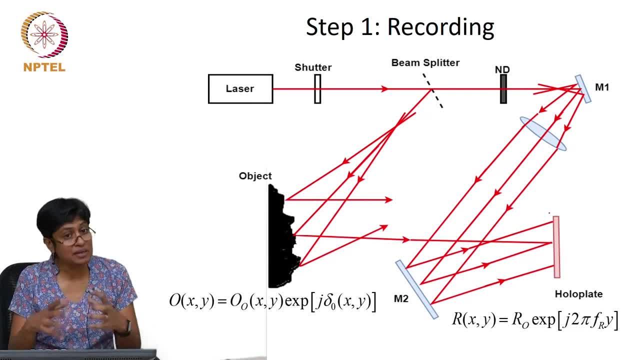 So when light is incident, a chemical reaction is happening, and that reaction varies also depending on the intensity that is on. So it is not only sensitive to light, it is also sensitive to the amount of light. ok, So that is why you have a shutter over here. 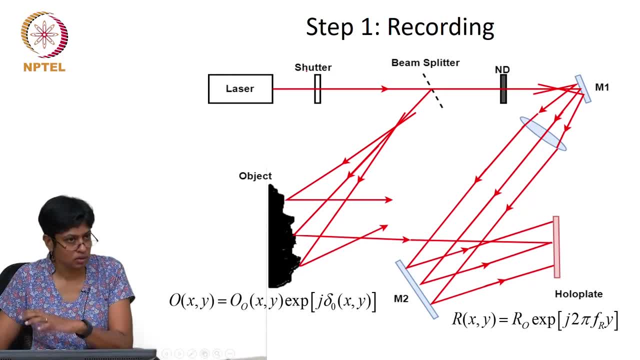 Why did you shut your system off? Because you need to have a lot of light to block or protect the hollow plate is and until you want to expose it. This ND is actually a neutral density filter. it just cuts the intensity of light. Why do 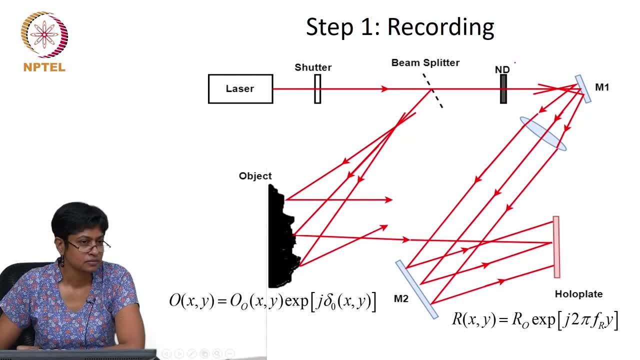 we have this here To help with the visibility. you want the fringes that are recorded to have good visibility. that means they are seen well. the modulation depth is high. In order to do that, the intensity of both these beams must be as close as possible. one is scattering of an object you would not. 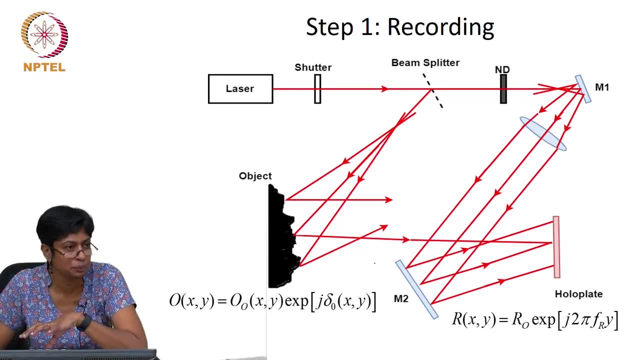 be surprised if you said that is the weaker beam reaching the hollow plate And therefore you have- usually will have- a filter here that just uniformly cuts the intensity of light. It is usually a variable filter. you can change how much you cut depending on how much gets. 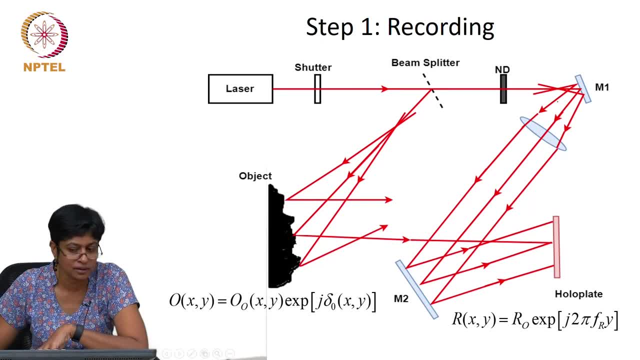 reflected of your object, of the type of object you are looking at, And therefore you are cutting your losing light in this arm so that the intensities in both arms are closer in value. ok, And that interference pattern now gets recorded. you Now I have written out expressions here. this is the expression for the object wave. 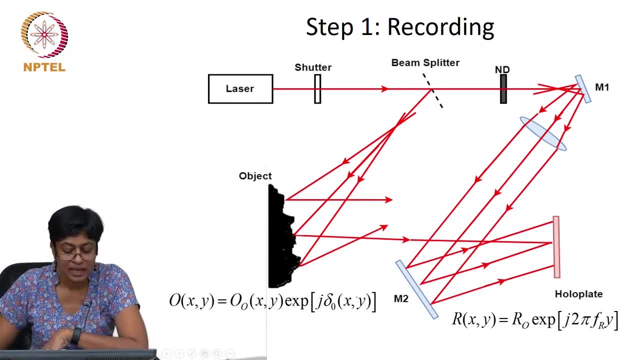 it has a certain amplitude. that varies laterally, It has a certain phase. therein lies the information. I do not know what that is, So I have just represented it as delta naught, or again. it varies laterally, So it is a function of x and y, The reference wave, on the other hand. 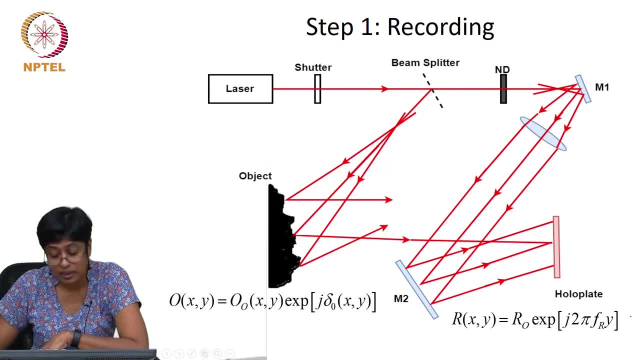 of course also has an amplitude, r naught and a phase, but here I can be more specific about the phase, because this is a known beam. So this expression 2 pi f r y means I have now got a plane wave that is tilted, and it is tilted in one direction, which is why I 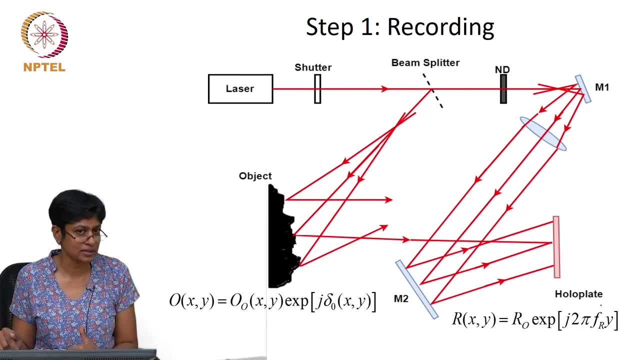 do not worry about the x axis here, I worry only about the y axis, and that f? r is related to the tilt and the wavelength of light. So though I have Similar expressions for both beams, object and reference, with the reference I can write out a specific expression because that is the known beam. ok, So that is the first step. 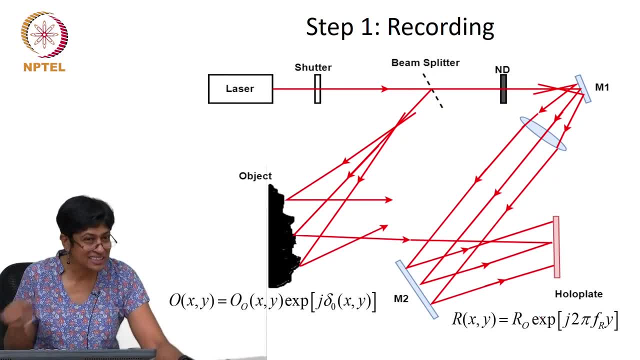 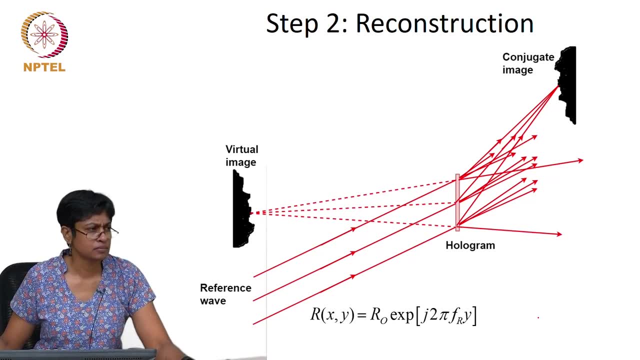 So what happens at that hollow plate? Somehow I have to capture the interference of these two beams. Why should a lens? So his question is: why should a lens? Why should a lens? So his question is: why should a lens? 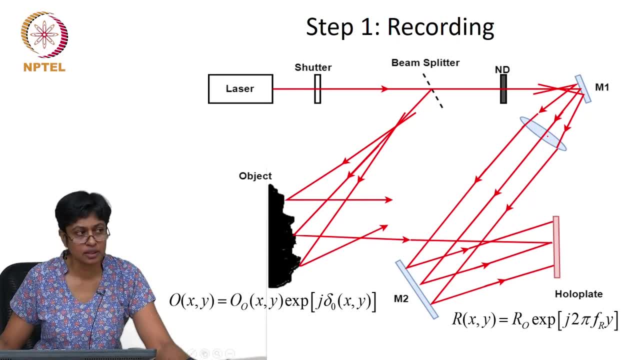 Why does not this converge? Why should it converge? Does a lens always converge Only if it has parallel beams on it? First of all, this optics is put into the system. So the mirrors and optics are put into the system only to indicate you may need optics. 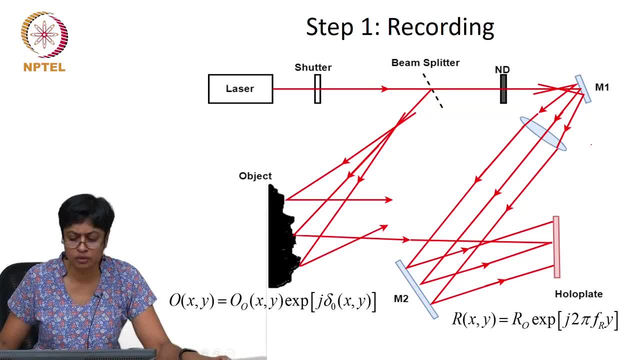 here to change the size of the beam. ok, Do not go by the scale or you know the size of the beam. Do not go by the scale or you know the size of the beam. You may have to change or position, but a lens converges to focus if you have a parallel beam of light. incident. 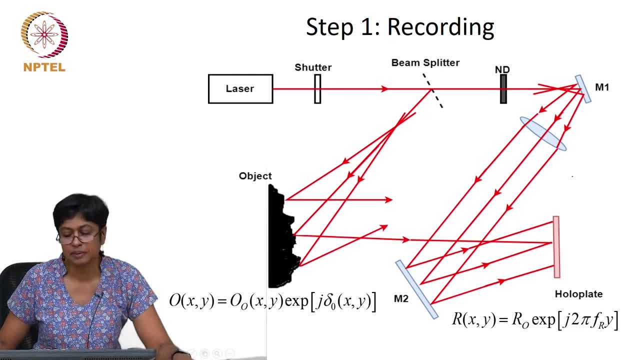 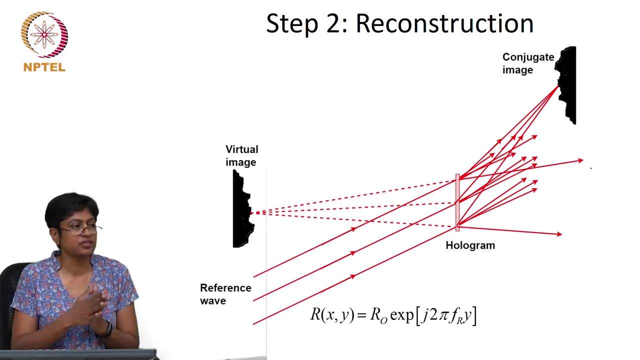 otherwise it does not right. but do not worry too much about what is happening over here. Anyway, I have, yeah, ok, Now, if somehow this interference pattern is stored on the hologram, the way the reconstruction happens is that you will now you remove all. 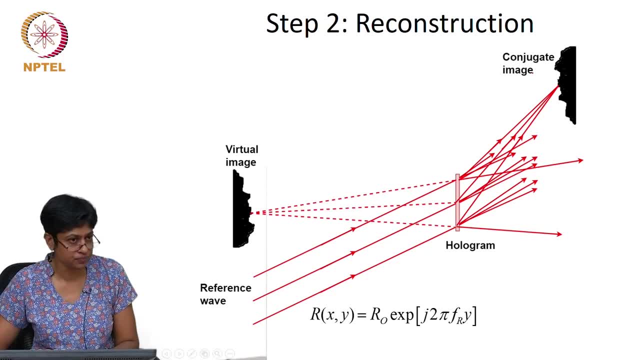 the rest of the optics. So all this optics that was here is gone. the object is also gone. What you do is you have the hologram and you illuminate it with the same reference wave. ok, Now, when I say same reference wave, I might 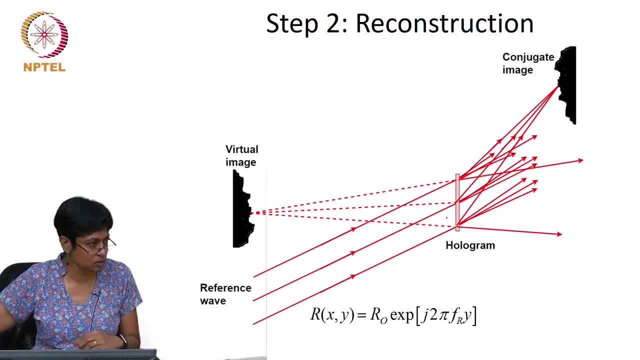 be recording the same reference wave. So I am recording the same reference wave. So I am recording a hologram somewhere and doing the reconstruction somewhere else. So I cannot have exactly the same wave. What we mean by the same wave here is it is the same wavelength. 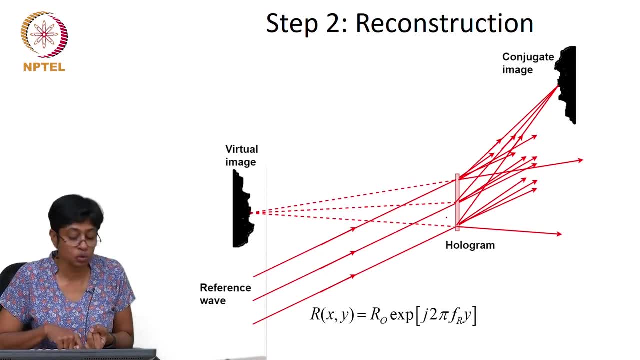 it is coming in at the same angle of incidence. So I can write out the, I can describe the wave in the same mathematical sense. that is what we mean by the same wave. So we have removed the entire setup that was used for recording and we now illuminate this hologram. 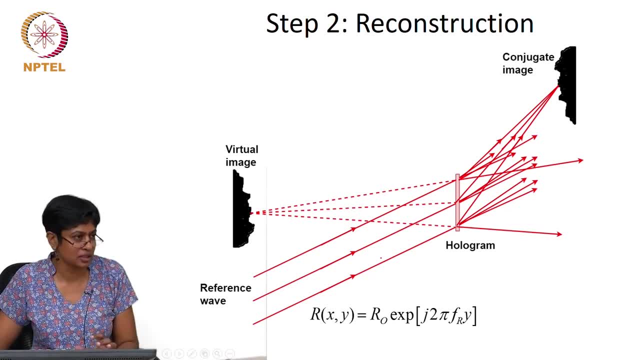 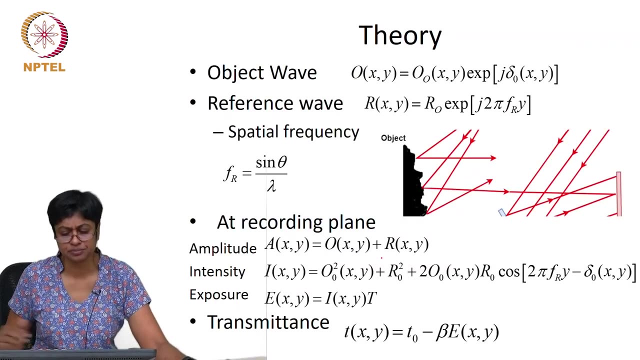 with this reference wave, ok, So this is the reference wave, and what happens in the reconstruction process is you will end up getting an image of the object, ok, And it is a three dimensional image of the object because it contains the depth information. So let us see how that happens. This was. 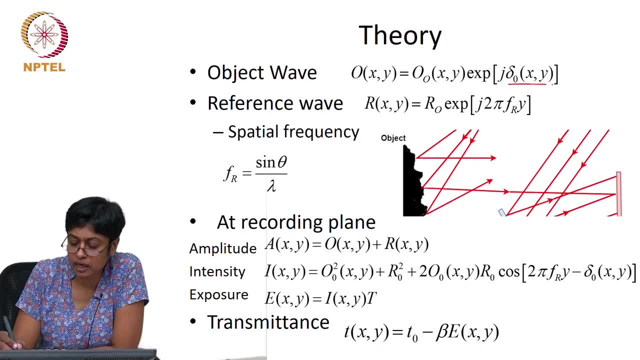 our object wave right. This was the unknown phase that contains the object information right In a hologram. So in a hologram. it is not necessarily that I want to get a value for delta naught of x, of y right I. it may not be that I need to quantify that, but I want that stored somehow. 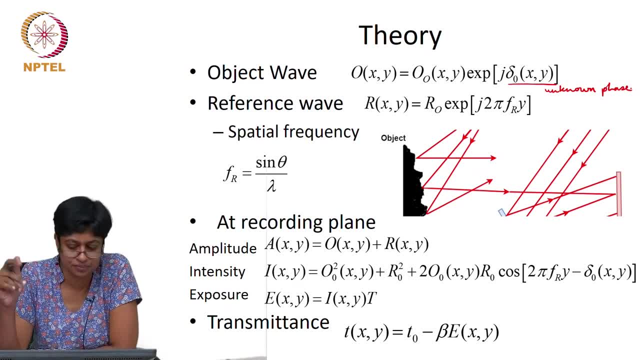 So that I reconstruct the object. that is the idea. This is a reference wave, this is known right And in fact, as I said, this f? r is a function of the angle of incidence, distance and the wavelength of the light, So these two beams overlap and the amplitude 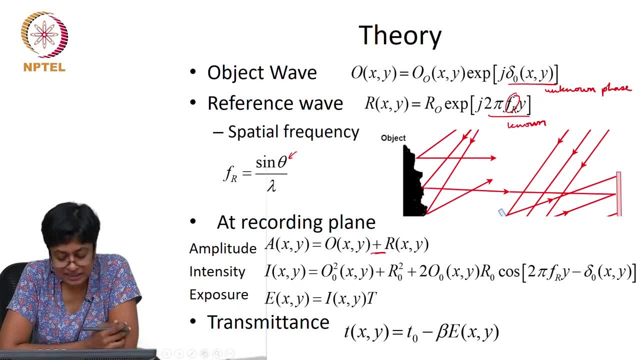 of course, is going to be nothing but the sum of them. the intensity, is going to be this squared, So the next term gives you the result of that squaring. I take this squared, So I have an intensity of the object beam. this squared, I have the intensity of the reference. 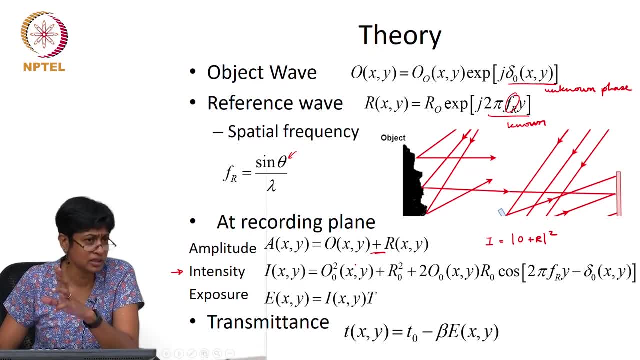 beam. This is exactly your two beam interference equation, because I a 1 and a 2 now and you had I 1 and I 2. that is what you see here. The next one would be the sum of the two terms that are O, star, r, the phase difference between them. 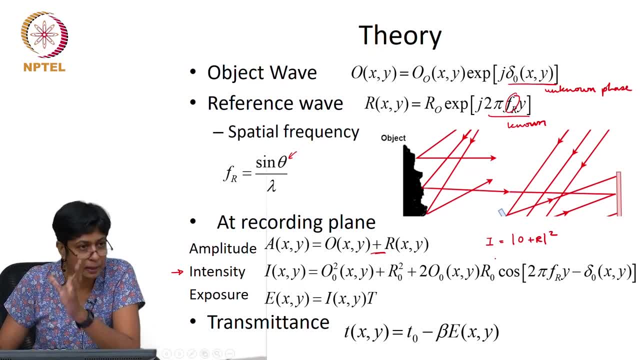 O r c Star, the phase difference between them. and if I combine those terms, I will get this cosine term here, that is: this is exactly your two beam intensity interference equation. ok, So this is the intensity that is falling on the plate which has this material sensitive to. 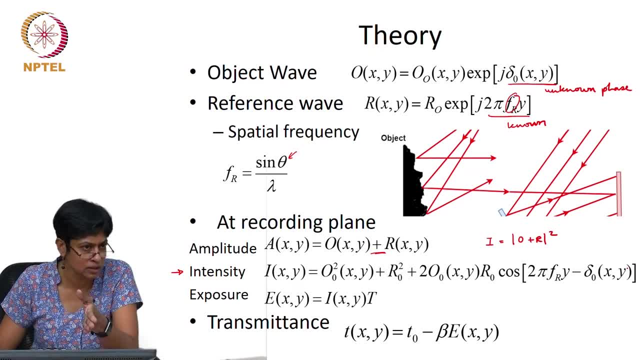 light and you can see the intensity varies across the plate. What is it a function of? It is, of course, a function of the original intensity, A function of the original intensities, but it is also a function of the phase difference. everywhere You know, let this light be incident on the. 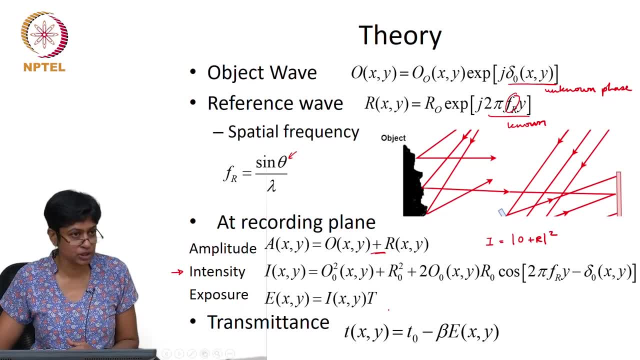 plate for a certain period of time, t. So that is the exposure. So the exposure is this intensity. I into the time t and we looked at what happens when you have a optical element with a certain transmittance right. We said, if I take the light out of this plate, when 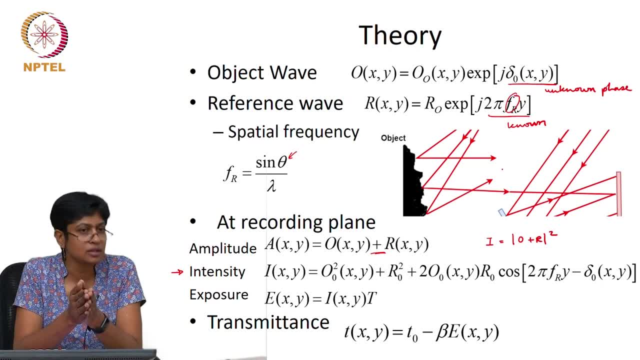 an element. every optical element has a certain transmittance. that means you have a certain beam of light incident on the element and then, based on the transmittance, it is going to have a certain behavior after the element. By exposing this holographic plate, you are 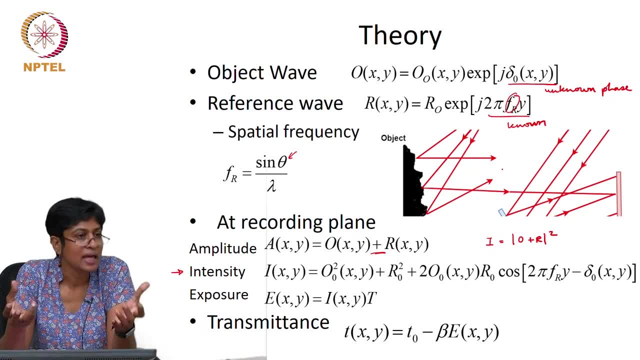 changing the transmittance of that element, and you are changing it in accordance to the intensity that is falling on it. That is how you are storing that phase information, because the intensity that is falling on it is a function of the phase right. So you are creating. 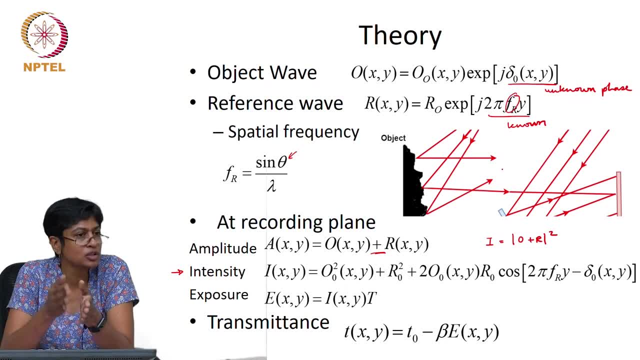 a transmittance. How are you creating that transmittance? You are creating a transmittance based on the phase difference between these beams. ok, So the transmittance ends up being So something like this, where you can consider: T naught like a DC transmittance, maybe the 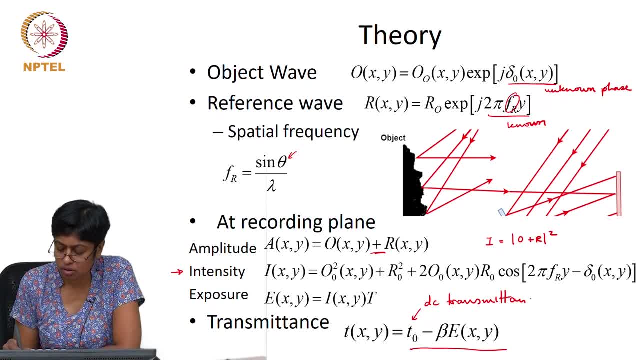 plate throughout will cut out 10 percent, So it is not. it should have been perfectly 100 percent transmittive, but it is not, So everywhere some amount of light is lost. So that is this DC bias: everywhere, irrespective of the location, it is cutting out some of. 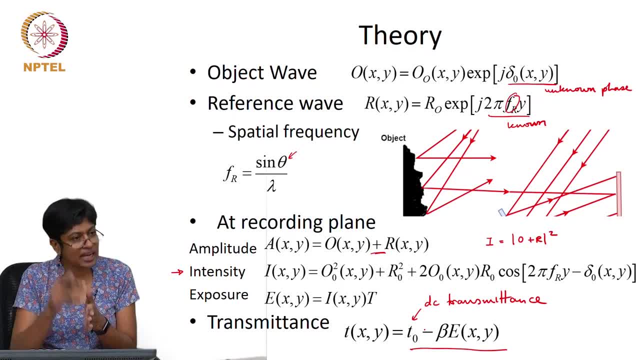 the light And then the transmittance. Ok, Ok, Ok, Ok, Ok. So transmittance varies location to location as a function of this exposure, and this is to do with some of the properties of the film that is on the holographic plate. So there, 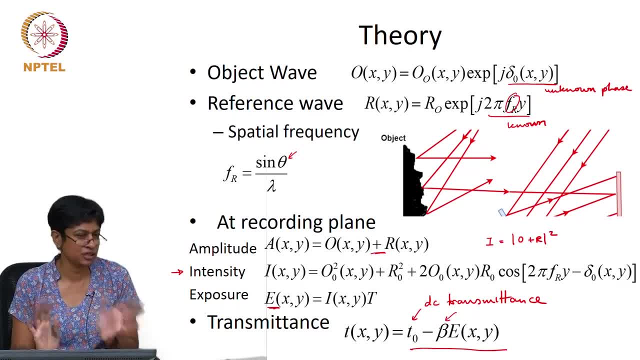 is some film which has these chemicals, and so that beta is a function of all of that. ok, as well as the development You have to actually this plate has to be. it is very similar to the old film technology, So it responds to light you. that is the exposure part. So 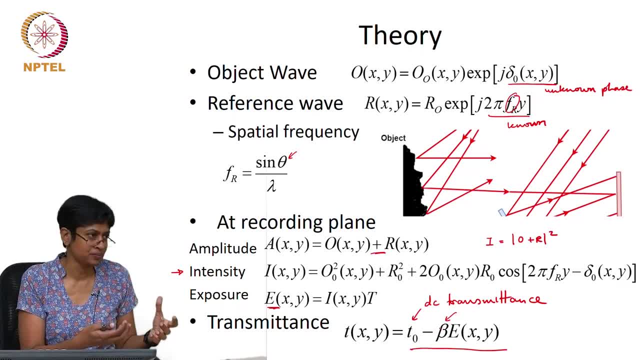 you actually have to put it into a chemical and develop it So that regions where the light fell you fix that and you remove other regions and then you are left with this pattern on the thing. So there is a whole process you go through but finally what you are left. 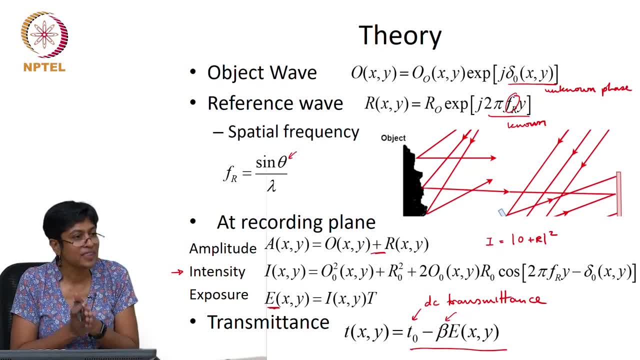 with is a plate with a certain transmittance that varies laterally, and that is a function of the intensity pattern that fell on it, which in turn is a function of the light. What is a function of the phase difference between these two beams? Is it clear till? 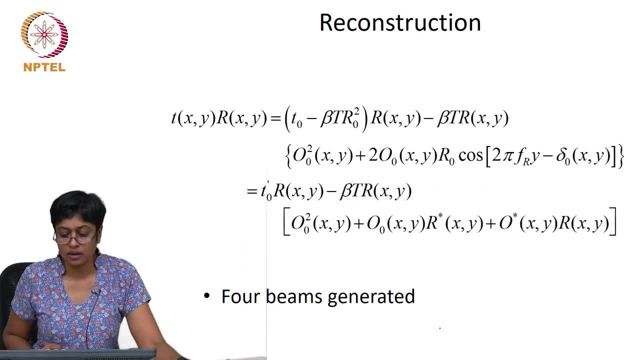 this point. So how do we do the reconstruction? Well, we know, if you have an optical element with a certain transmittance, multiply it by the incident beam to find out what happens after the element. So that is what we will do here: we and what is the incident beam. 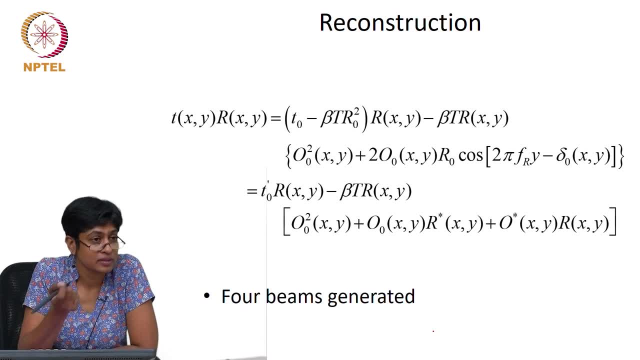 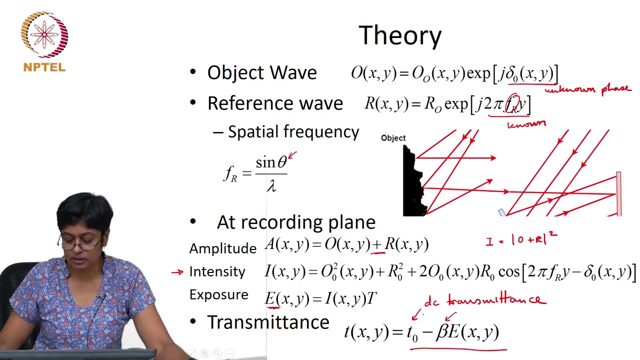 What does it have to be for a hologram? It has to be the reference wave. So we take this is an hologram, or the transmittance of our hologram, this is the reference wave. multiply them and remember this is the expression that we had, So this substituted into this. multiplied by the reference wave, is going to give. So What is this? The reference wave? Ok, So there has to be a reference wave, So there is the reference wave. So what happens when we have the reference wave? So 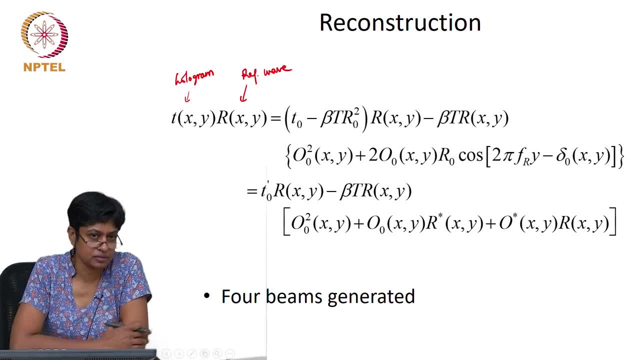 me these different expressions. ok, Just take a moment and look at them right. It is just taking the transmittance and multiplying it by the reference wave, and since the transmittance has every term of the interference pattern in it, the resulting transmittance has a number. 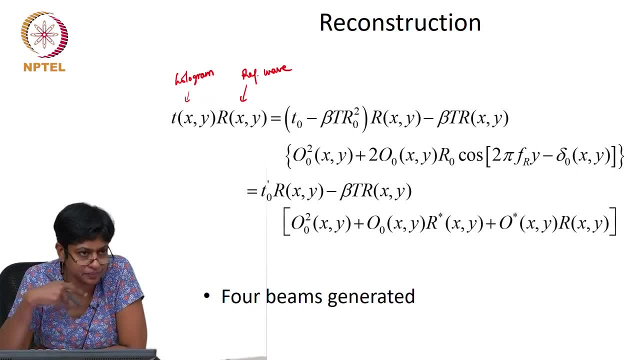 of different terms in it. It is not a single term. It turns out in fact there are four terms. Now if I take, you know, I write something like this: ok. 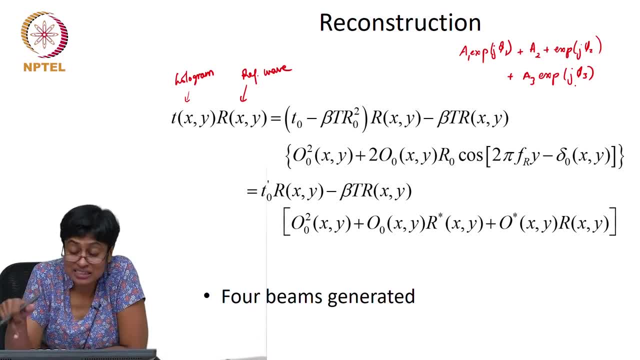 That summation means that I am looking at the combination. oh sorry, this is not a summation. the summation between each of these terms means that I could consider each of these to be a unique beam. it has a certain amplitude. 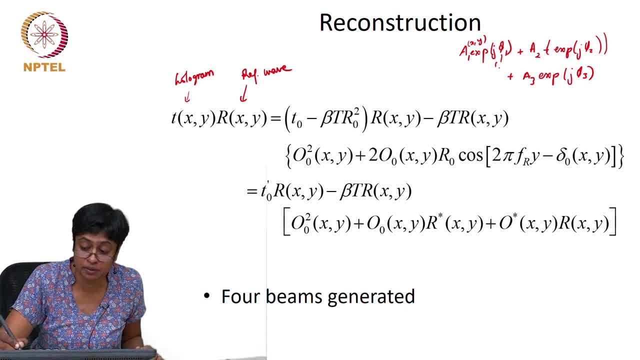 that amplitude may be a function of x and y. the phase may be a function of x and y, right, Each of these I could consider as a beam. When I say take this beam plus this beam plus this beam, it means all three beams exist simultaneously Buried in that phase. information would be information. 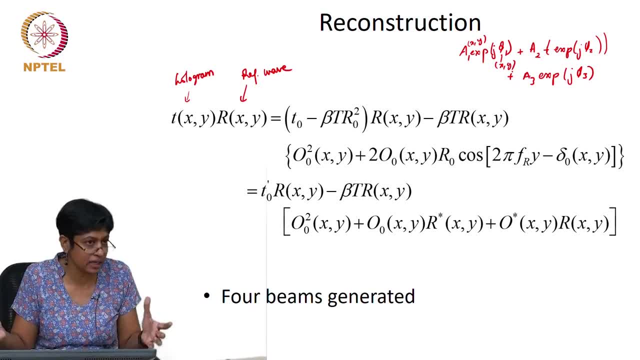 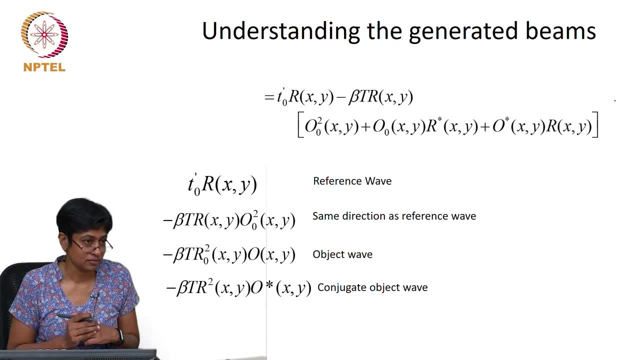 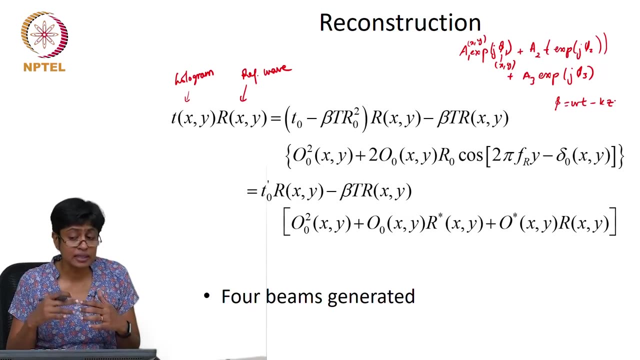 on which direction this beam is traveling. I have just put it as phi, but phi, remember, is omega t minus k z. it tells me the direction of travel. right, We might assume that these beams all have the same wavelength. Let us say I make no changes in wavelength, So there. 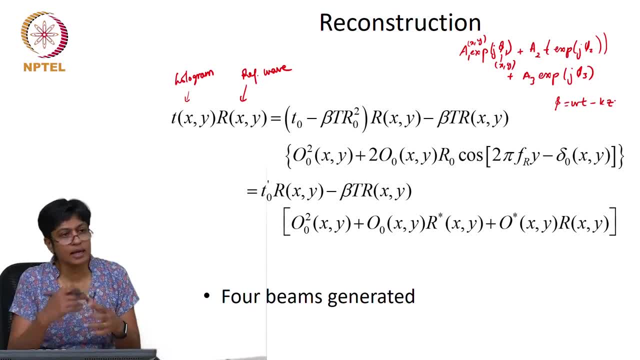 is: these beams are incident on something, they are reflected. and now I am looking at these different beams and, let us say, the wavelength does not change, but the direction can change in each case, right? So buried in this is the information about the direction I can clearly see there is. 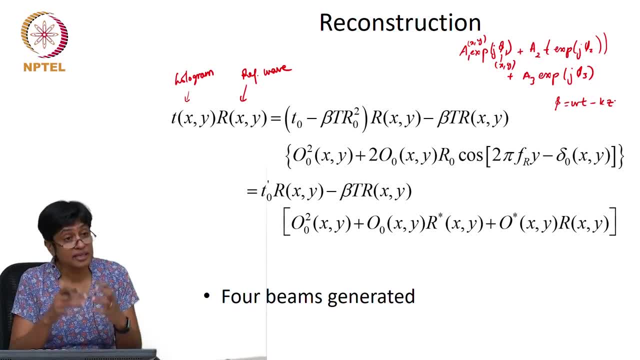 an amplitude variation. When I say this plus this plus this, I am then looking at a space in which these 3 beams exist, though they may be traveling in different directions. So I am looking at that combination. So what happened when I multiplied the hologram with the reference beam Since its transmittance? 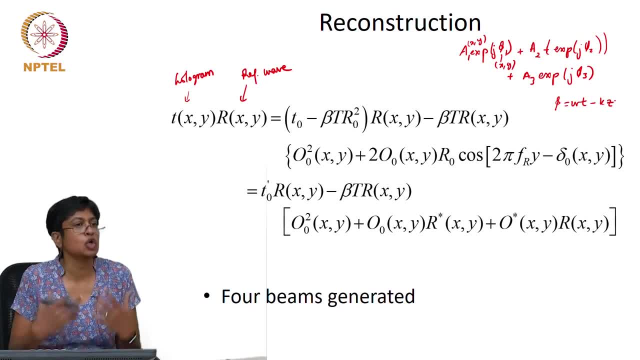 was the sum of several terms Rightə. So, including whatever the reference beam there have been, which are you taking at least terms? the multiplication also resulted in the sum of several terms. Optically, what does that mean? It means multiplying or having the reference beam. incident on the hologram. 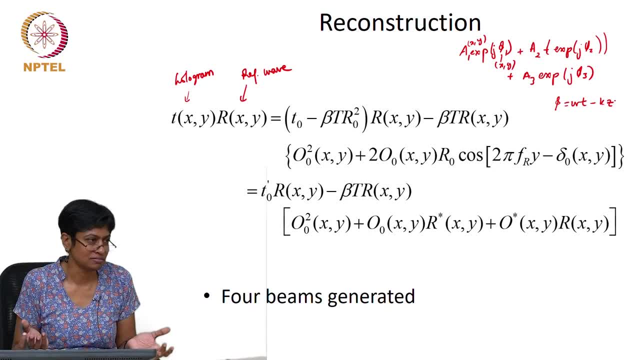 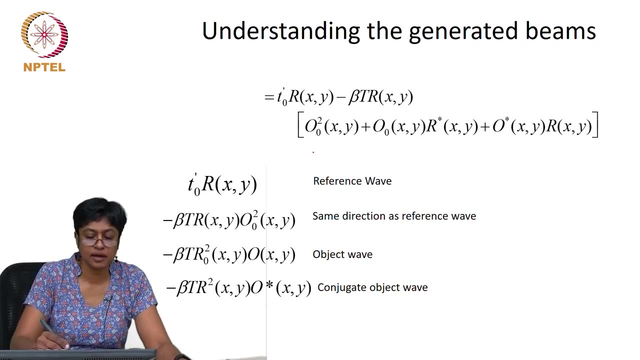 generates a number of beams. right, and there are four terms. I can quite confidently say: generates four beams. ok, What do those four beams mean? So this is our expression. right, You have this, you have this and you have this and, of course, this. ok. So if I look, 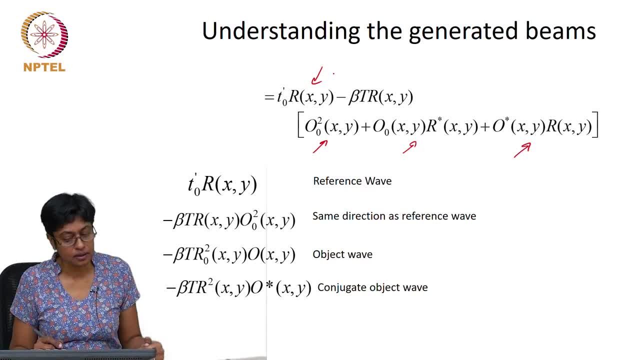 at them separately. I have, So these are the four beams. I have this, So these are the four beams. I have this, So these are the four beams. I have one beam, and how do I make out what each beam is from this multiplication of so? 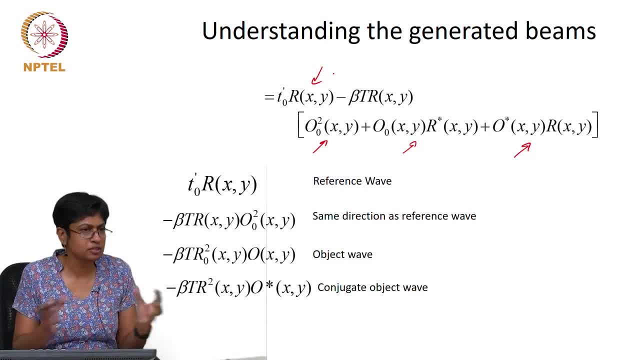 many parameters right. Which one of these gives me amplitude information? which one gives me phase information? How can I tell which of these, what part of each of these, will give me phase information? You all agree, the multiplication results in these four beams right. So if these are beams, 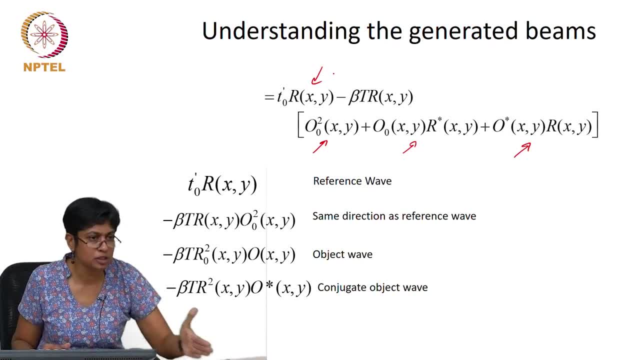 then I must be able to say: this is the amplitude of this beam, this is the phase of this beam, and if I can say this is the phase of this beam, then I can say this is the direction this beam is travelling right. So, in each of these, which term will tell me what is a phase or has the phase within? 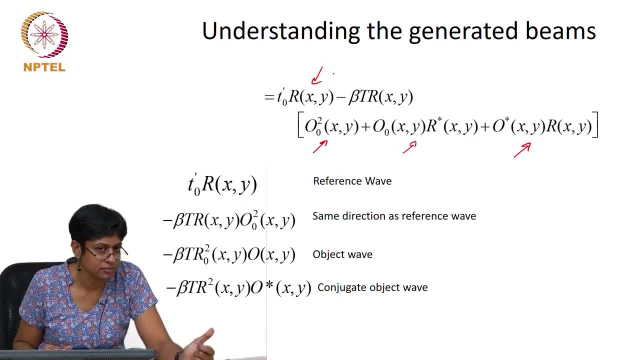 it. Can I tell, or can I not tell, The last terms? You say the last terms, Last two terms, Last two terms, meaning Each one of these is a beam. So this is beam number 1,, this is beam number 2,, this is 3,. 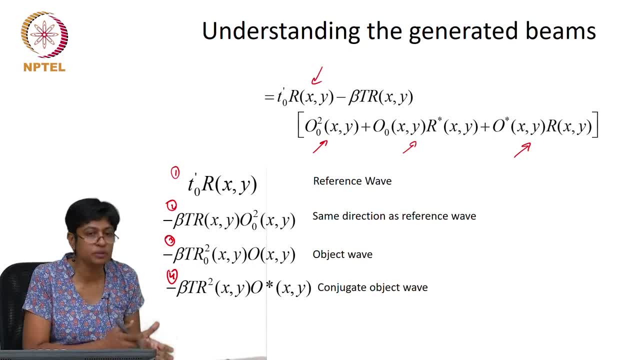 this is 4. that means each one of these has an amplitude and each one has a phase. So what is the phase in each one of these? The phase has to have that exponential something, term, right. and where does that exist? It does not exist here. it will exist in this I have. 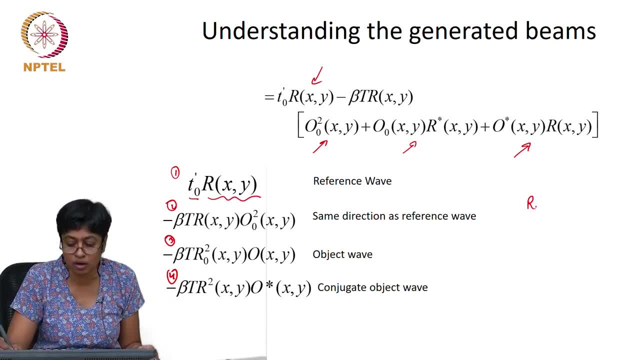 written. this is capital R x of y, but you know that is r, naught exponential, that whole term right j of 2 pi f r y, right, that is what we had put: 2 pi f y, right. So the phase lies in this, in the second term. where does the phase lie? It will again lie here, because 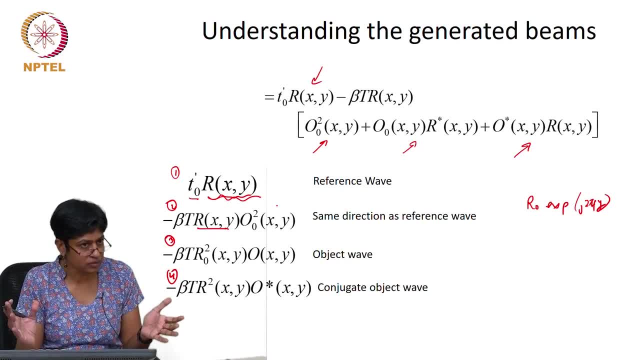 the o naught squared, the phase has been multiplied out of that. that is a pure amplitude term, and in the next one, the r naught squared, the phase is no longer there. So the phase lies in this and in this case the phase lies here. ok, 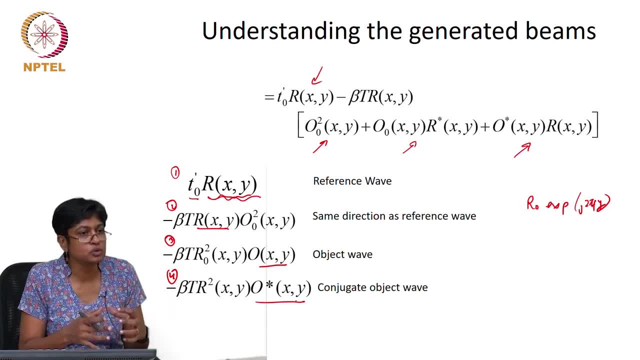 So the rest of the terms contributes to the amplitude of the beam in each case. So you are generating 4 beams, but you are not generating 4 identical beams. You are not even generating 4 beams with identical amplitude. You are generating 4 beams with each of these 4 beams. 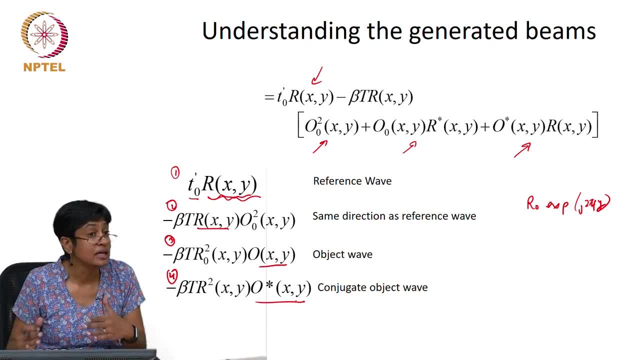 each one having a different amplitude, each one having a different phase, travelling in a different direction. ok, So of interest in terms of phase is the highlighted ones in each case. ok, For the first beam, what is the direction it is travelling? It is the same direction as the reference. 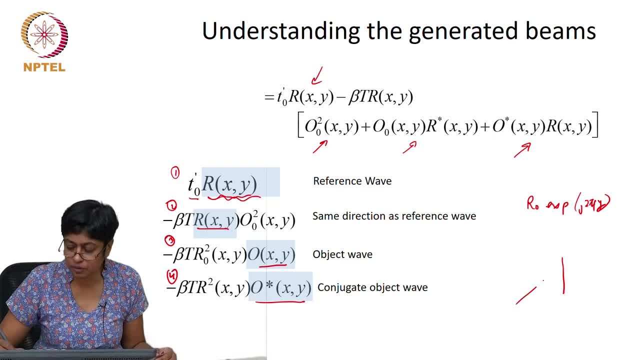 beam. So on this holographic plate you have the reference beam incident and then you have a beam that continues in that same direction, right Unsurprisingly, its amplitude is not the same as the incident because it is interacted with this plate with this varying transmittance. 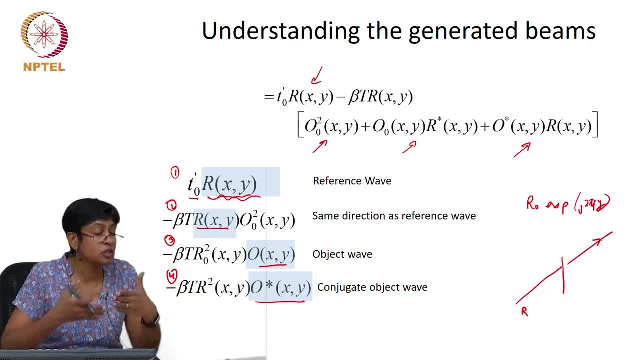 all of the light that was incident is not going in the same direction. If all of the light incident was going in the same direction, there would be no in light or energy left. So there is no energy left to go in any other direction. I should not, strictly speaking. 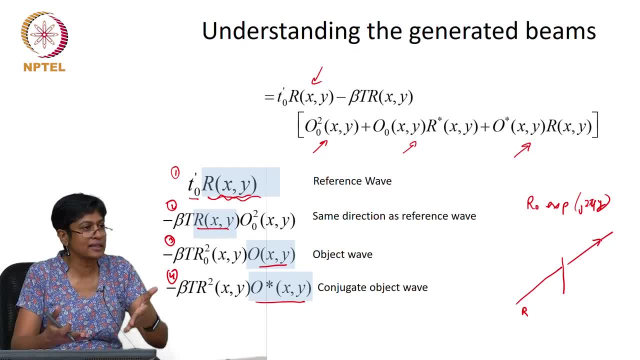 have any other beams then Then I would just say: I have a beam of light that is incident and this plate does nothing to it. it is as if it does not exist and the beam continues on the path. The whole point of that hologram is that somehow it imposes information on 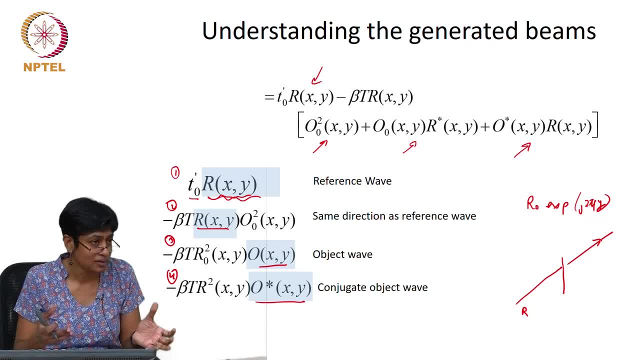 the beams, and we can see beam number 1 is not giving us any information, So it arises from the nature of the setup, but otherwise is useless to us. ok, So where which beams or which beam carries the information that is useful to me? Well, it must be the beam. 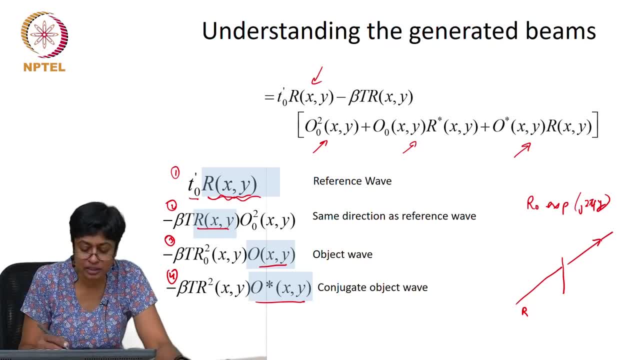 that has the object phase in it. and you can see, there are two beams, there is one which has this and one which has this. ok, What do you think? a conjugate object? how would So the object, The object wave, carries, the object information, the object phase. If I take the conjugate, 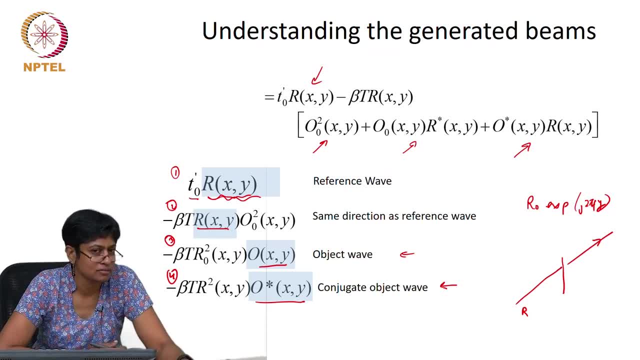 of that. how would that look like? How would I perceive it differently? Phase is negative. Phase is negative. you have mathematically told me what happens. So I have a beam, is e power, so exponential J phi. and then I take 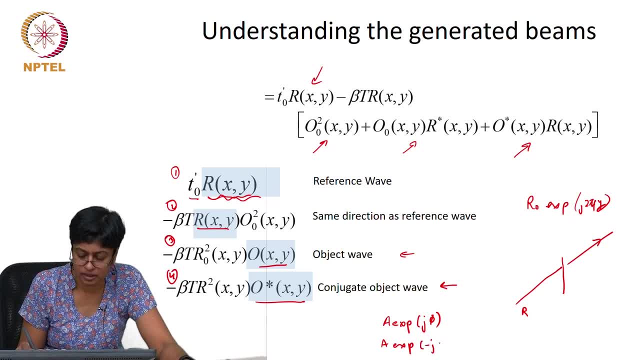 the conjugate, and I say that is exponential minus J phi. ok, and you look at these two, how will our eyes perceive this as different? Will we see that difference? Finally, what is our eye respond to? Intensity of phase? So we cannot tell. 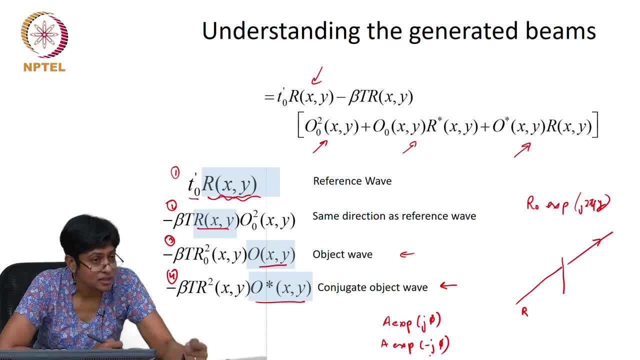 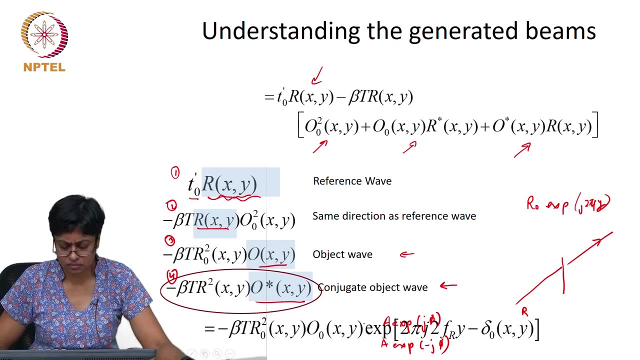 the difference. right, But what is the difference? The difference could be actually in whether something is here or something is here, could be some difference like that, but we might not be able to tell. ok, So the beam of interest then to us. I can. 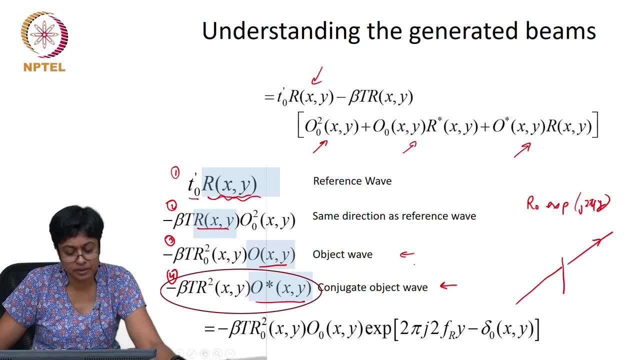 look at as this beam- number 3, it seems to be the beam of interest, the object, And if I write it out explicitly you can see it contains the phase of the object. So that is the phase we are interested in, but the phase term does not have only the phase. 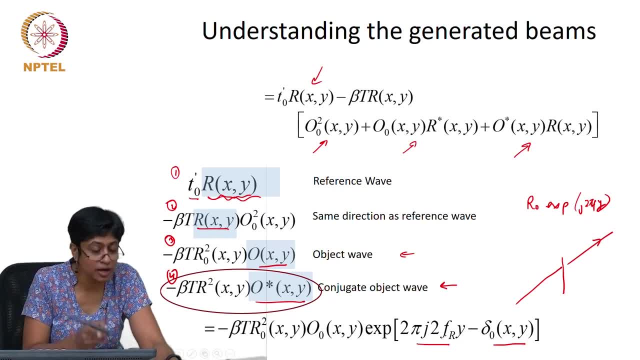 of the object. it has this phase Because it is r naught squared. there is an extra 2 here. So how has this changed the phase of the object? The phase I am interested in is this: And yet in the exponential I have this phi 1 and this phi 2.. I want phi 2, but I have 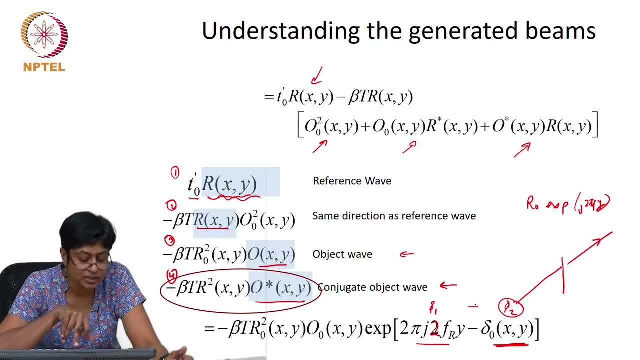 phi 1 minus phi 2.. What is that going to do? How is this beam now different from what I want? What is adding a phi 1 do? What will it do to a beam? Let us say I took this beam and I somehow remove this phase from this beam. What would I be doing to this? 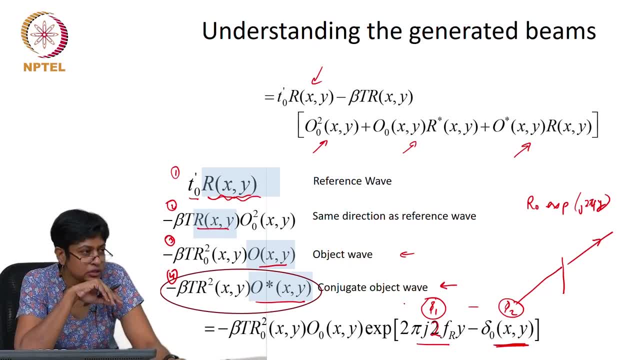 would I be doing to the beam? I do not affect the amplitude, but I remove this phase. what would I be doing to the beam? What does adding a phase there do? In fact, when we wrote out the expression for the reference beam, this, I said: this f is a function of. 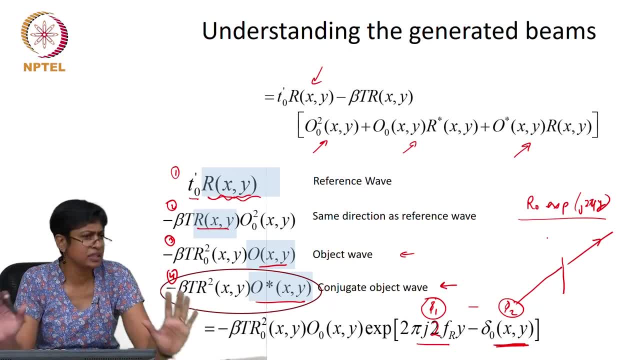 the angle of incidence and wavelength. So we are keeping everything simple, we are saying everything has the same wavelength, so wavelength is not affected. So what could this phase? by removing phi 1 or adding phi 1 or introducing phi 1, how am I changing this object beam? 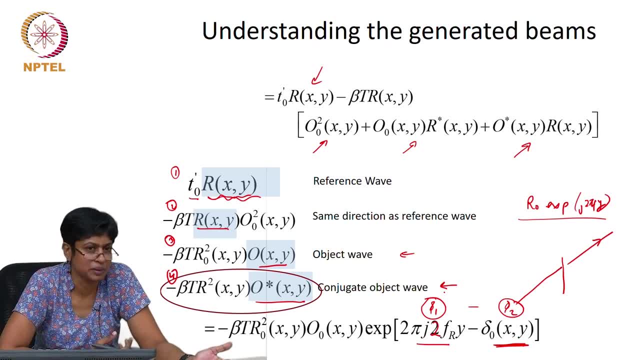 You are just changing the direction of the beam, right? If it has the original angle, then you say that the beam travels in the same direction. I expect to see it in that same path, in that same axis, but by adding this phase I have just changed the direction of. 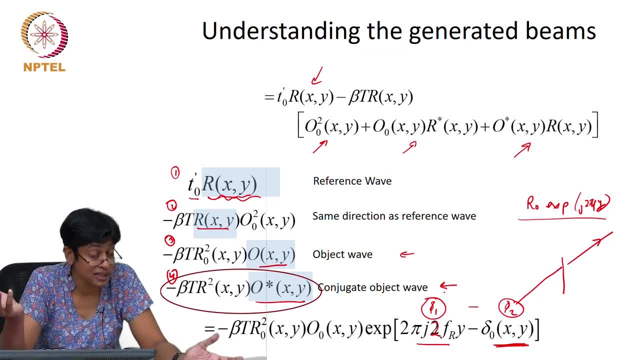 where the object. So what was our entire goal of starting goal with holography? We wanted to capture, Capture the phase of an object so that we could reconstruct that object and get the full three dimensional view. What this expression is telling us that, yes, I can do that. I generate. 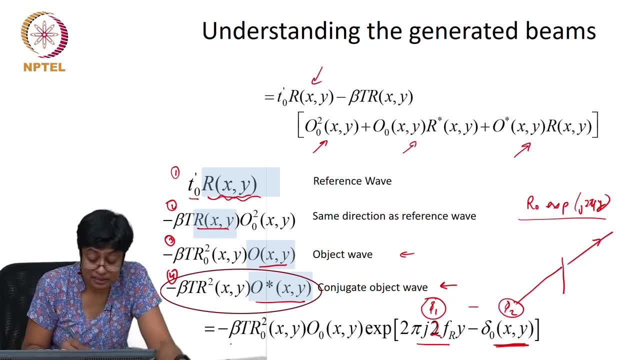 a beam that has the object information in it. this tells me there is some scaling factor that is multiplied right. So the object beam amplitudes are this, but I multiplied throughout by some scaling factor. So that does not matter. this is going to have a certain scaling. 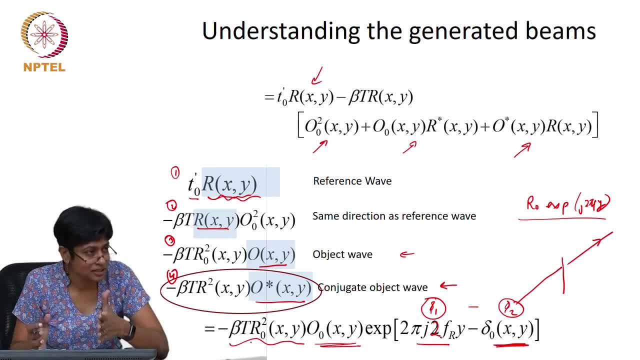 factor and, in addition, that object beam is travelling now in some direction which is different from the original object beam. but that does not matter. my goal is to get the object beam. I live with the fact it is in a different direction. What controls the direction? 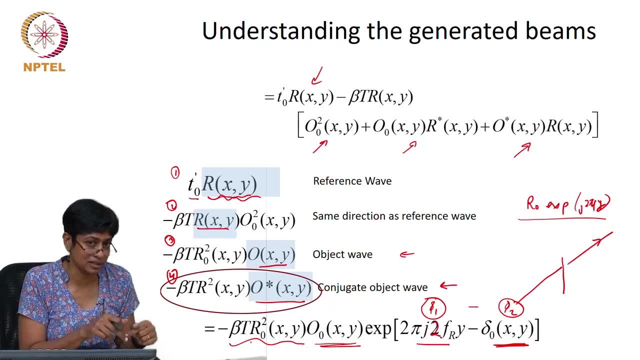 The original reference beam. The original reference beam angle will control that direction. So I have some play there. I can change that angle a little bit. but there are some reasons why I would not change that angle too much. but I could in this recording set it up to have a certain angle So that 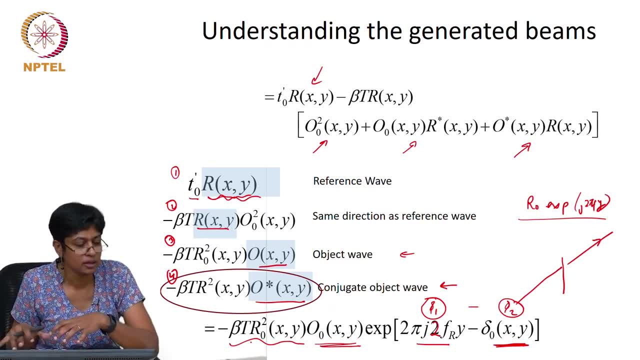 I control where the object beam happens. ok, So what were the steps? again, We did recording where we took the light scattered of the object and interfered it with a plane reference wave. that intensity got transferred to a plate sensitive to light and modified the transmittance. 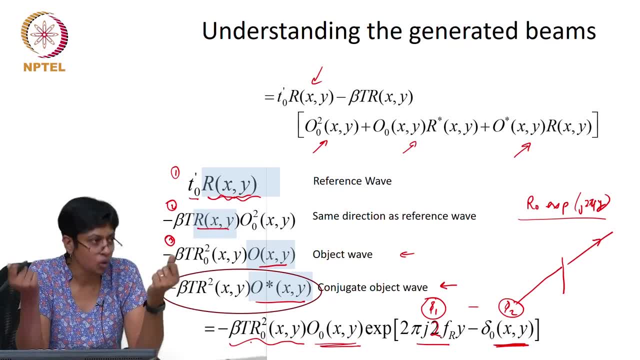 of that plate. That plate is now what we call the hologram. We illuminate the hologram with the reference waves, with the same angle, and we see we generate a number of beams, One beam clearly not useful to us. it is the reference wave and in fact, if you look at the second beam, We also see that another beam is not used to us. that is the reference wave. So if you look at the second beam, if we look at the second beam, the reference wave, and these two beams are not used to us, it is the reference wave. So 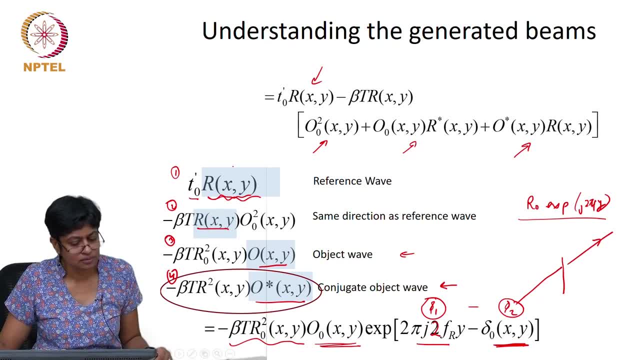 beam. this is also a reference wave, right. Both of these travel in the same direction. their amplitudes are slightly different, right? So these two are of no use to us. The second two seem to have the information we want. the difference between these two is the directions. 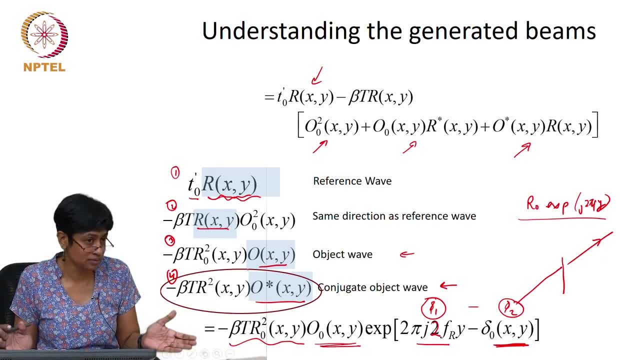 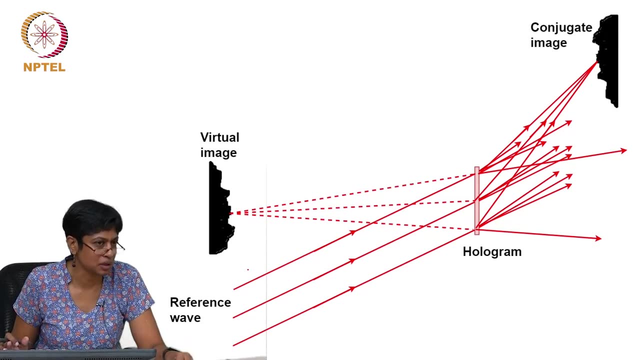 they travel, So they are separated, which is good, right. So it may at first glance appear like you have created two objects, and in a sense you have. but it turns out one is a real object and one is a virtual object. So when you 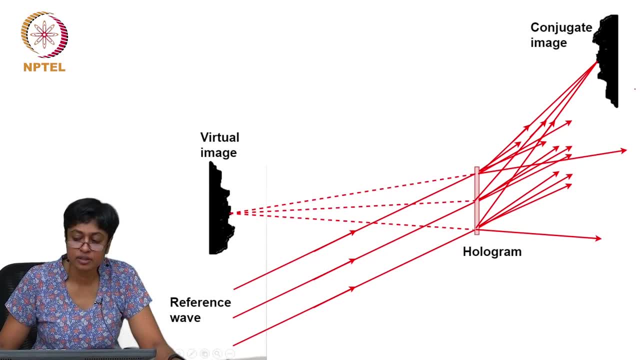 illuminate, you will have light that converges, forming the. this is the conjugate beam, So it is not in the same position as the original object, but the light that converges is not there. The image is actually formed by light focusing and coming to that point. So if 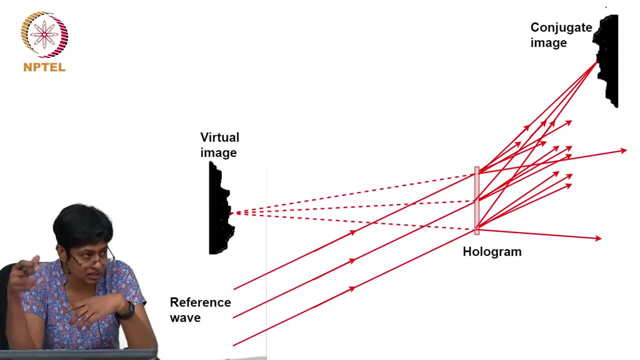 you put a camera there or a screen there, you would actually see the image. The second image is a virtual image, So that is light going off in some direction. but if you were to trace back, it would look as if it were coming from the original object position, right? So 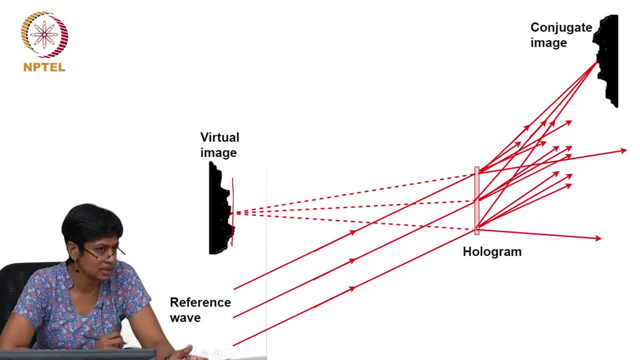 if I actually put a screen here, Here, I would not see anything because there is no light actually focusing to that point. but if I looked from this direction, my eye lens would look at that light and it would reconstruct as if the light were coming that point, and so I would see the virtual image. 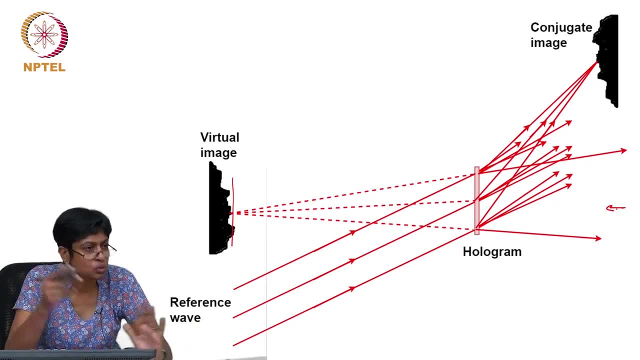 ok, So four beams are generated. two are following the direction of the reference beam, One converges to an image that I could then see, So photograph, make a two dimensional image out of, and the other one gives me a virtual image. So the four beams correspond to these four different directions. ok, So in a nutshell, 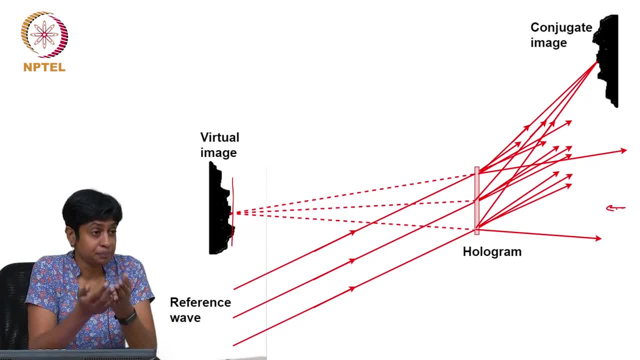 that is holography. ok, By using interference, by adding this reference beam, you are capturing and storing the phase and then for reconstruction you are able to get out. So the thing is, we say conjugate image here. how do you think this image is different from image you see? 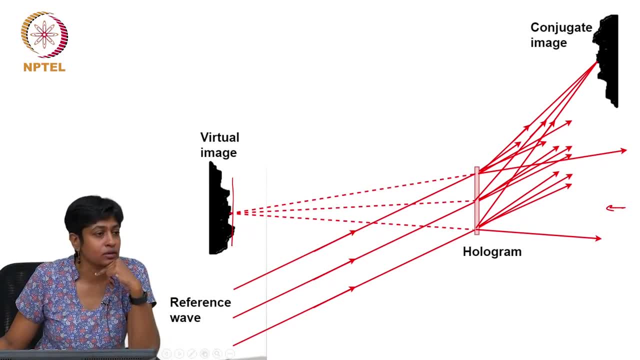 in a magazine or on your TV screen or on your phone? How is this image different from an image taken by a camera? I mean, we have said it, but what could you do with this image different from what you do with your phone when you? 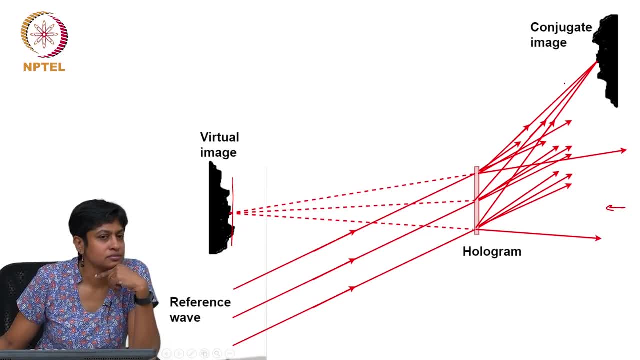 look at something on your phone, You can actually perceive depth. You could walk around this image and you would get perspective. you would see something from this side that you do not see from this side. right, You would walk around, depending on how that hologram was recorded. 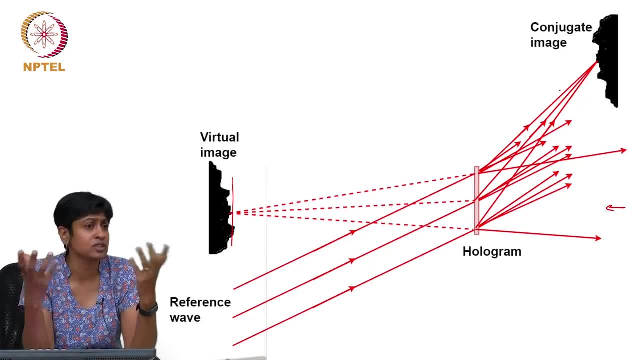 The image was scattered from all around and there are many different ways of recording the hologram right. So in tomorrow's demo, which you will see in the physics department, they will show you holograms and you will be able to walk around and see how it is very. 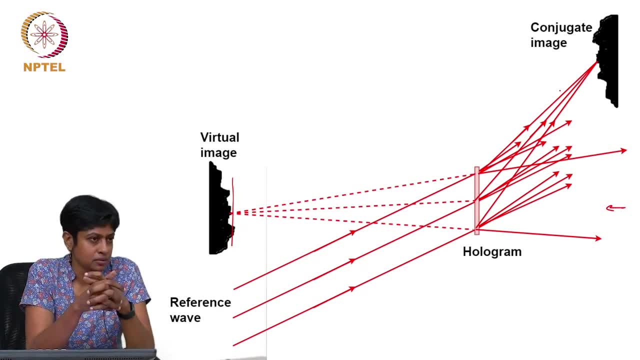 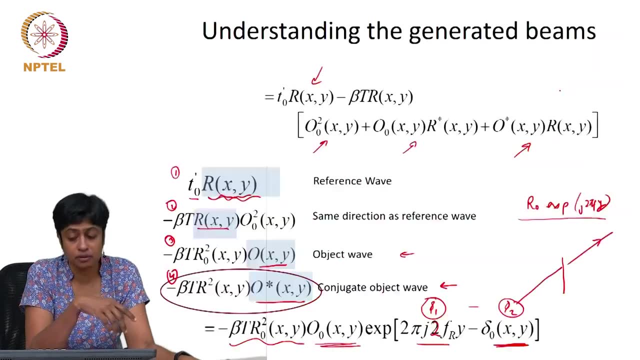 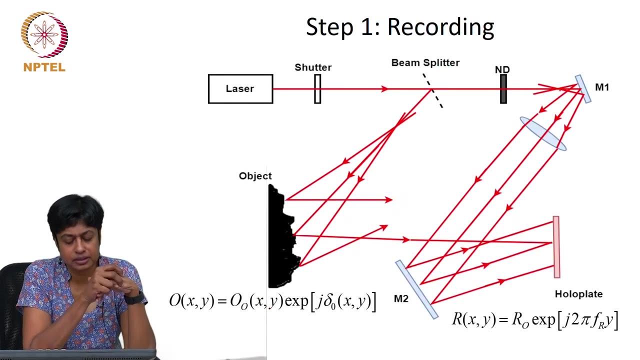 different. ok, There is another big difference between image taken with a regular camera and the image taken with by holography. So if we look at this recording process, I have a drawn all the rays here, As I do all the rays it would. 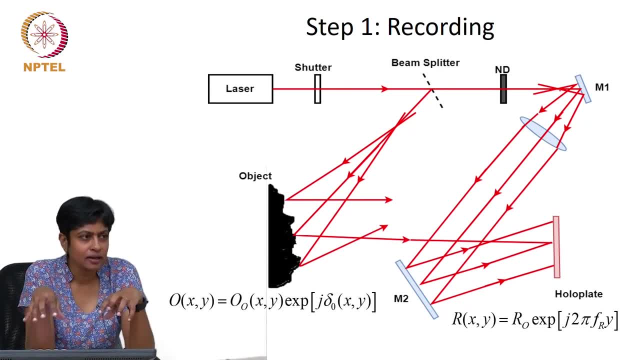 be just too messy, right? Can you tell one big difference between this recording process and a recording of a regular, of an image taken with a regular camera? What? that is one very big difference. In fact, we spent the first 6 weeks doing geometric optics and saying some one sentence. 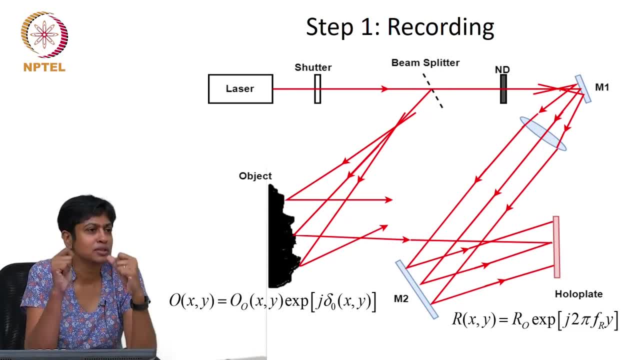 I went on saying, we use a lens to ensure that dash, dash, dash, dash. What is a big difference from the light coming from the object in this case, compared to how we capture light from an object when we are going to take an image with a regular camera? 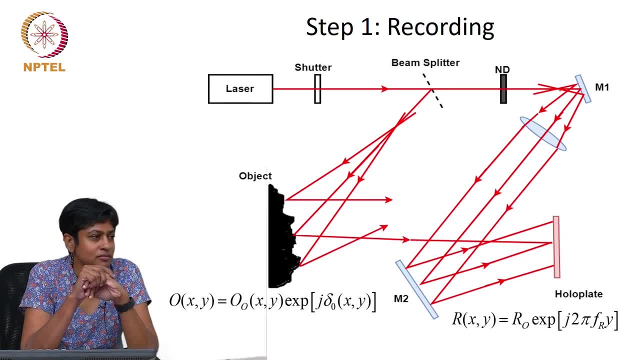 First of all, there is something missing here which I could not. I mean, I cannot take an image in a regular camera without that right. I need a lens. my regular camera always has a lens. What role did that lens? when did we say we had an aberration? 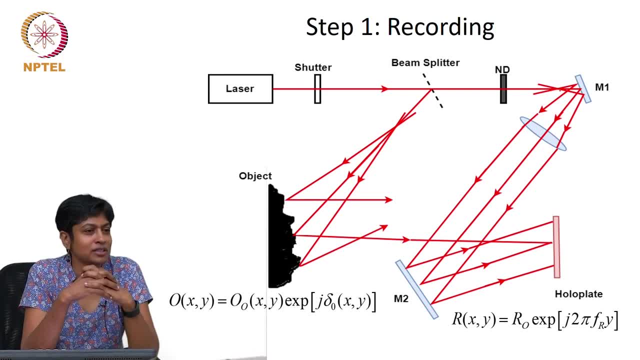 Geometric optics. right, Remember that topic that we briefly brushed against. Off axis because of lens. ok, these are three useless answers. ok, Off axis, big lens, because of lens. and Mathu, I did not even hear your answer. Give me hope. what was your answer? 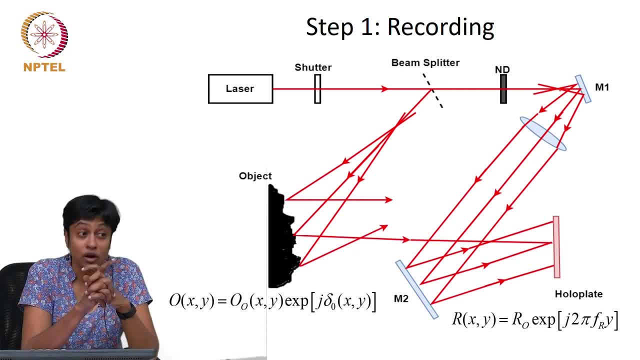 Not focused in the lens. Ok, So you said: not focused, There is no lens, There is no lens here, there is no question of focus here, right? So how is it that I am getting the information that I want? That is even. that is not even the question I wanted to ask you. I want to ask you something. 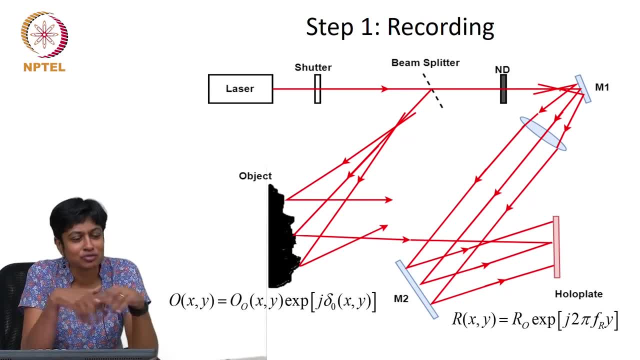 else, but we need to answer this first to You- did not actually describe the object used in the case. There is. This is it is. So I am saying the only optics I may have left out is optics to make it large enough. 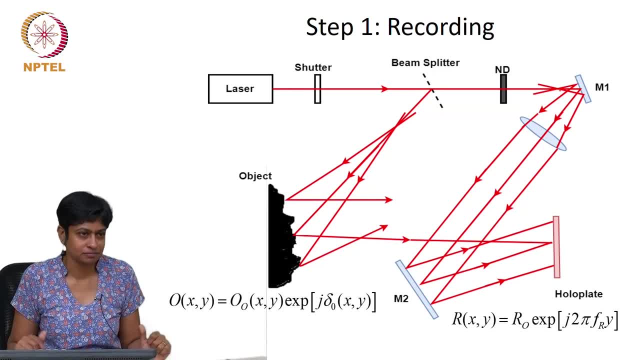 to illuminate the object. ok, The light that is scattered of the object is what hits the holographic plate. That might get rid of chromatic aberration. but that is about it, Ok, Thank you, Thank you. Thank you very much. 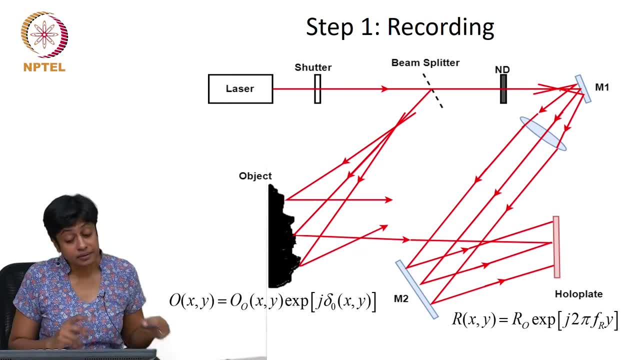 That is that present. So all in the, in a conventional imaging I used to keep doing this. I would say: let us say I am imaging a tree, then all the light from one point on this tree or one point on this object, this optical system has to capture all of this light and if it is a good system, 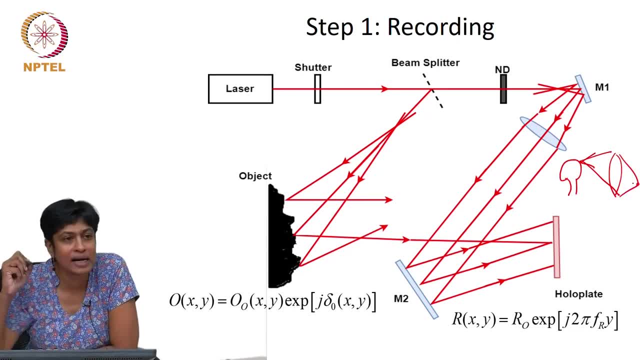 a well designed system. I am not doing that here. I am saying the light scattered of the object, all of the light scattered of the object, reaches this right, and that means light scattered. from this point, some of it will reach this, some of it will reach this, some of it will reach this. 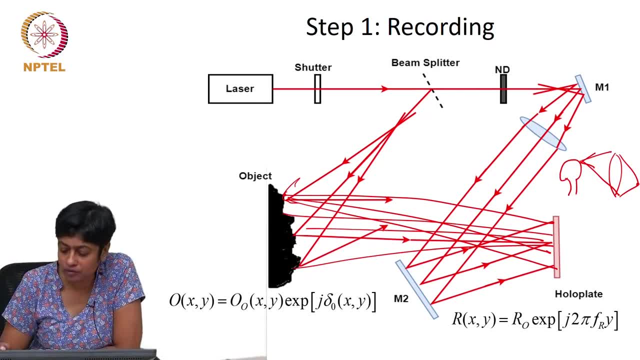 In my conventional imaging system all of the light from one point had to go from one point on the image plane. that is how we defined aberration. if it did not form one point, we said it is aberrated. Here I have removed that constraint completely right, because I am not capturing the image. 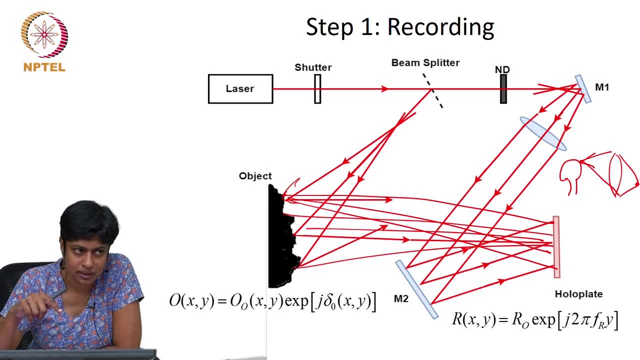 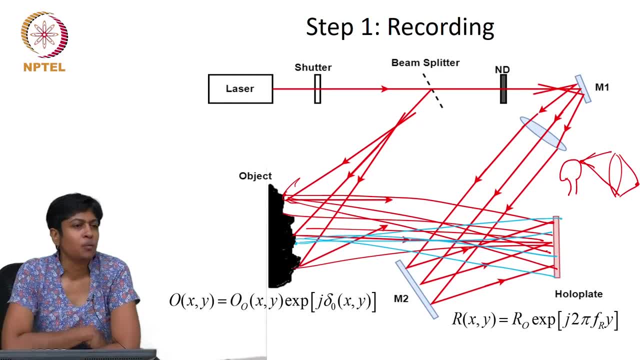 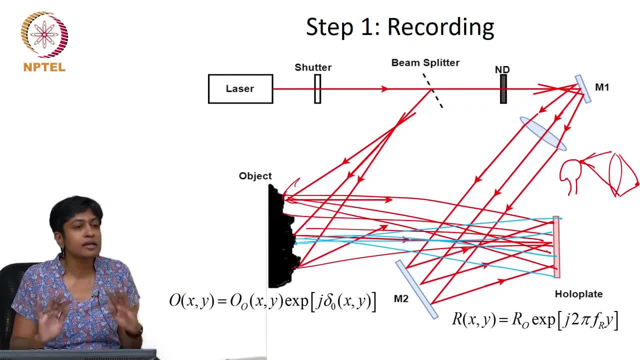 I need a lens to do imaging, and now you say I do not. holography is one thing I find a bit easier to understand When I do the maths, because with the maths I showed that the intensity is a function of these two beams, and one of these beams is the scattered beam that's going everywhere. 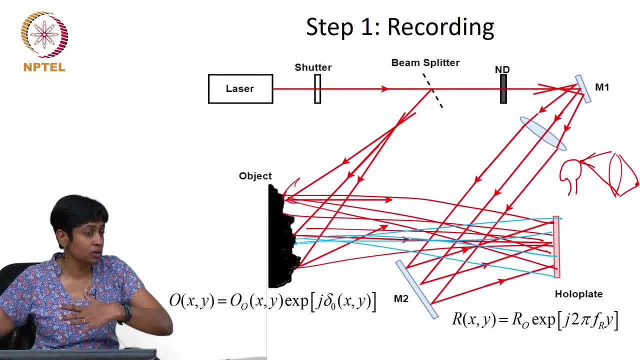 right, that transforms the holographic plate, and when I illuminate it, you. so you got four beams, of which some beams carry object information. So go back and understand, be convinced of the maths. the physics of it will follow right. But what is the advantage of the fact that light from one point is exists all over my 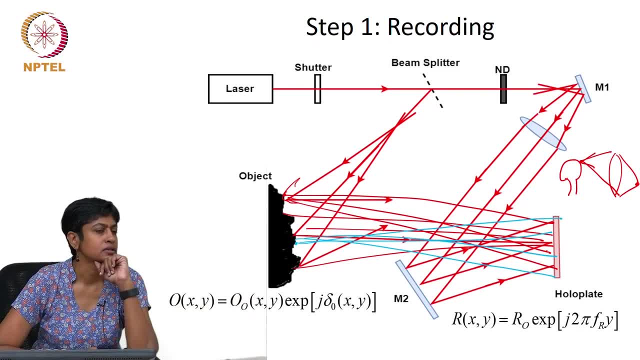 hologram. What is the advantage? in that It looks different from different angles. that is part of the holographic process. yes, yes, but what is the other? and what would? what would? So you will see this. tomorrow, he will show you a holographic plate. 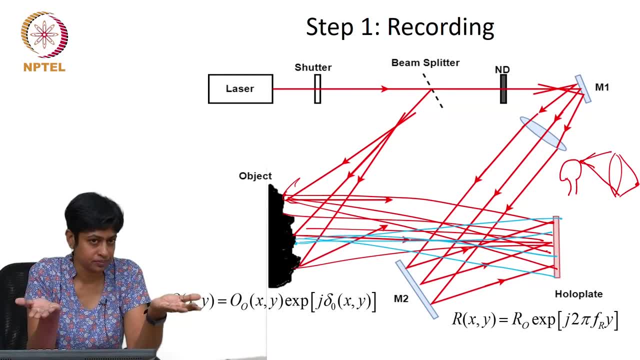 So if I give you a holographic plate and I give you a photograph, with the photograph, you look at the photograph and immediately know what you are looking at. right, When you look at the hologram, you do not have a clue what you are looking at. you will see. 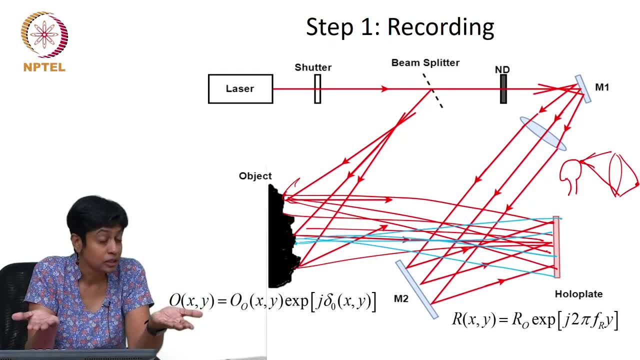 a fringe pattern or some weird noisy kind of fringe pattern So you do not directly see. you need that reconstruction process to see. ok, If I take my photograph and cut it in half, Have I lost information? cut it in half and throw away half the photograph I have lost. 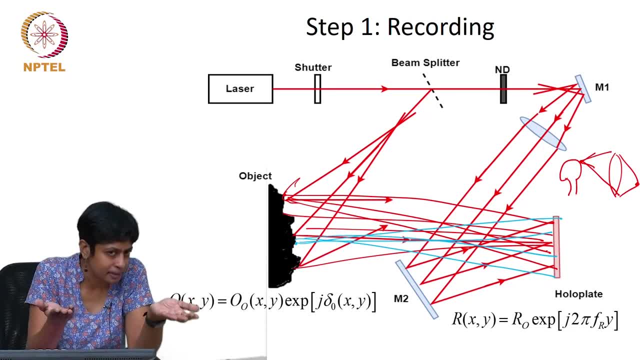 information right. If I take my hologram and break it in half and throw away half, have I lost information? I have not, because every point on the hologram contains information about every point on the object right. That is one big advantage, Of course, when I reconstruct. 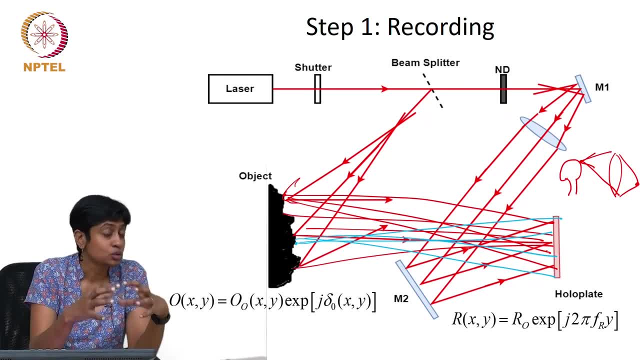 I am reconstructing with half a hologram, So if I could send so much light onto the system, I can only send half that light. So the intensity may go down, the brightness may go down because less light is taking part in the process, but the information about every point on the object is stored everywhere.